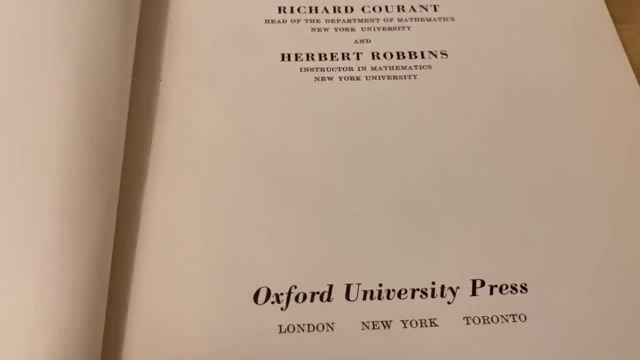 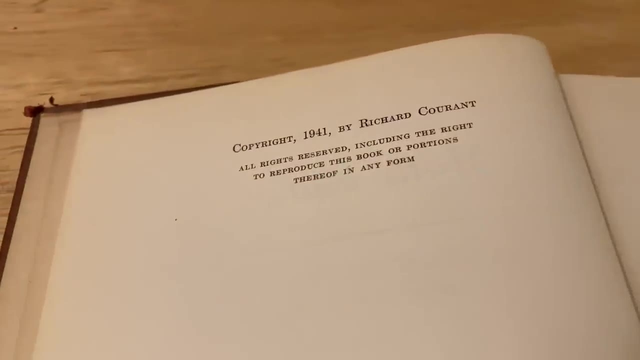 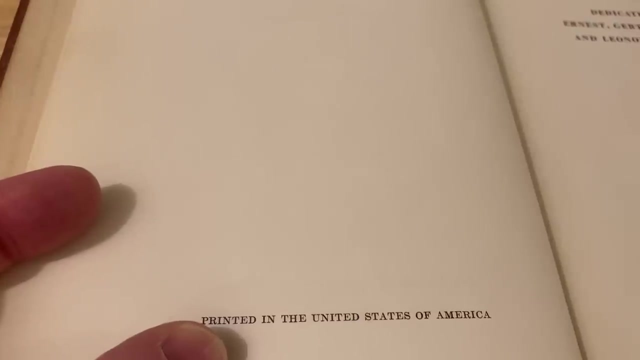 instructor in mathematics, New York University, Oxford University Press. Copyright 1941 by Richard Courant. And yes, this is the same Courant from the Courant Institute, So it's the same person after which the institute is named In the United States of America. Here are the dedications dedicated to Ernst Gertrude Hans and. 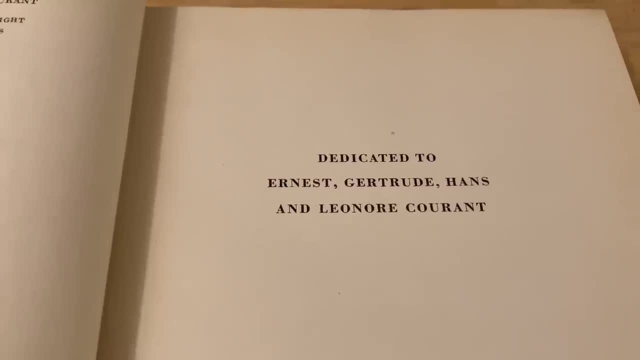 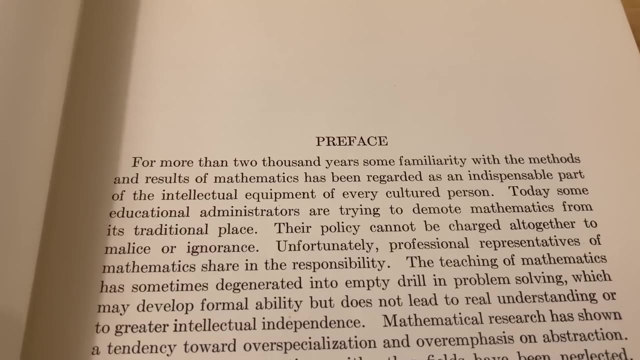 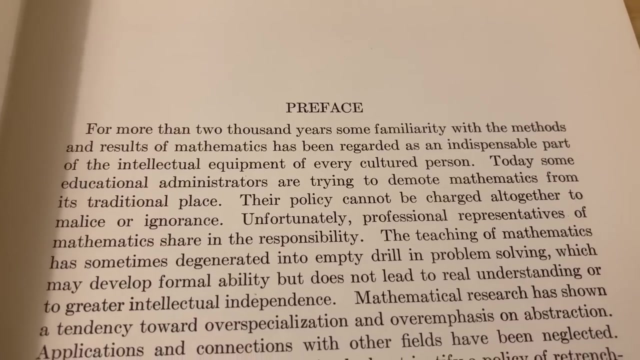 Leonore Courant I should mention. Courant was a German, American mathematician and he fled Germany in 1933.. Let's just read small bits of the preface. For more than 2000 years, some familiarity with methods and results of mathematics has been regarded as an indispensable part of the 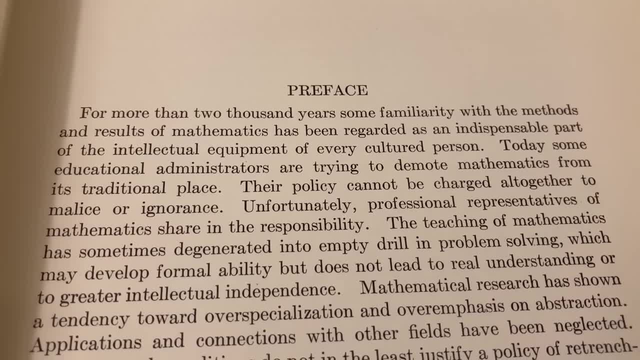 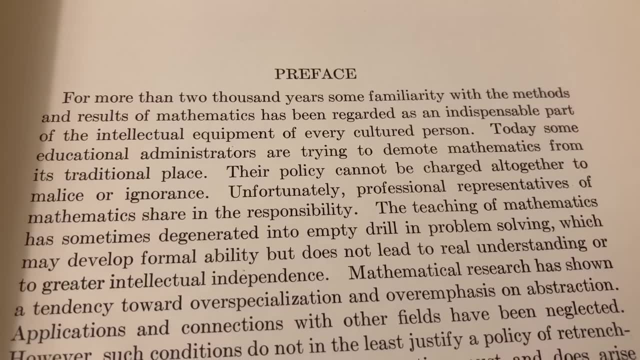 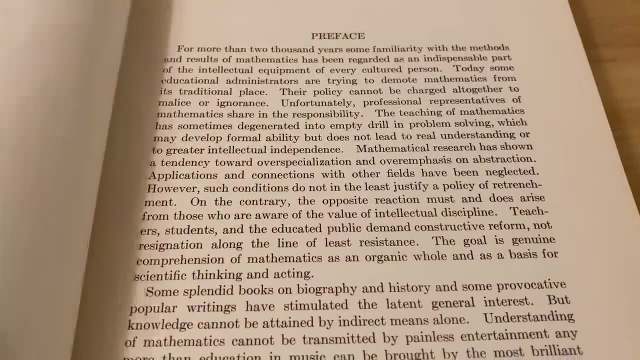 intellectual equipment of every cultured person. Today, some educational administrators are trying to demote mathematics from its traditional place. Their policy cannot be charged altogether to malice or ignorance. Yeah, very interesting because a lot of people have similar views today, And it's funny because this book was published so. 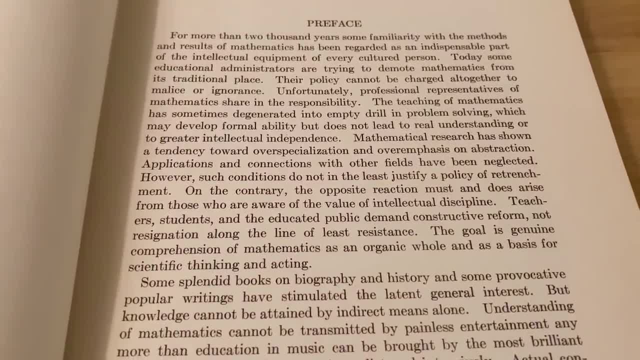 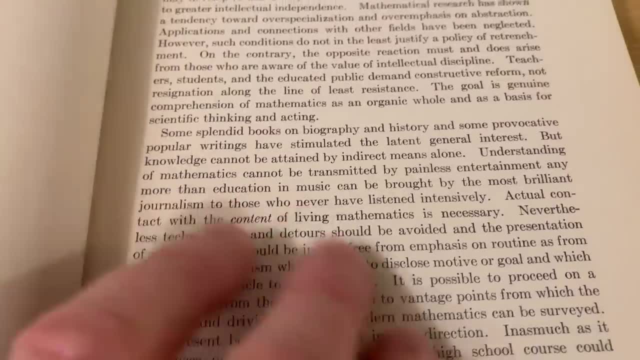 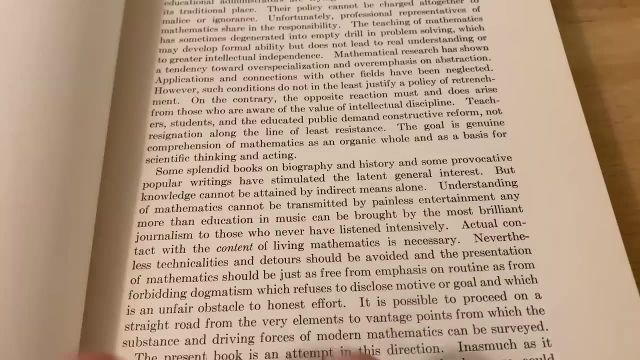 long ago, 1941.. So it shows that not much has changed. Actual contact with the content of living. mathematics is necessary, And I feel like that is the theme throughout this book. It's not a book on philosophy, It is not a book on you know why mathematics should be this way or that. 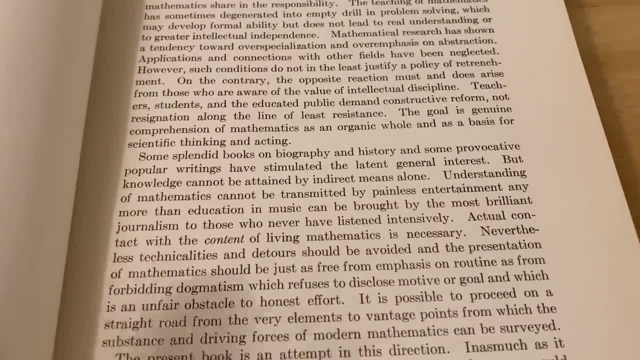 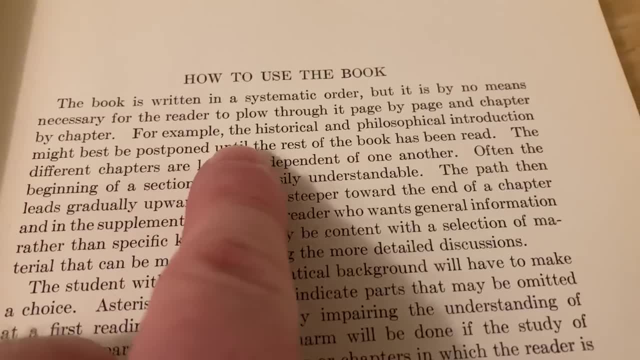 way. It is a book on actual mathematics, And Courant explains it in a brilliant way here He talks about how to use the book, And I just want to read one sentence to you. It says, For example: the historical and philosophical introduction might best be postponed until 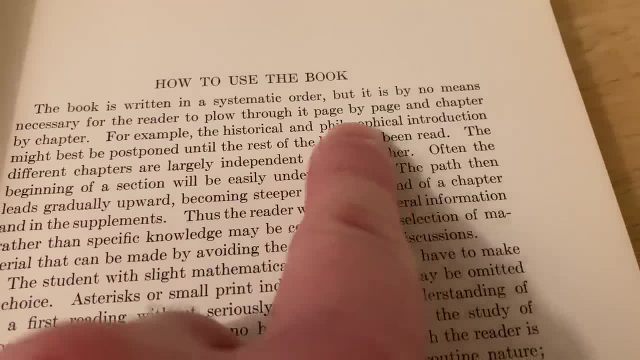 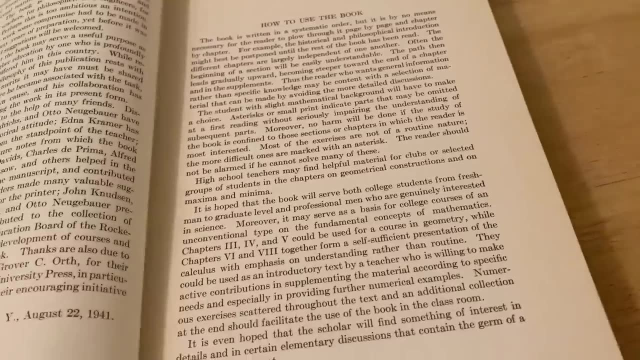 the rest of the book has been read. In other words, Courant is more interested in actual mathematics. I'm getting goosebumps because I've spent a great deal of time reading very, very, very interesting books on the subject of philosophy in my academicitei. I suits all that. And it's not a book on emotivals. It is not a book on 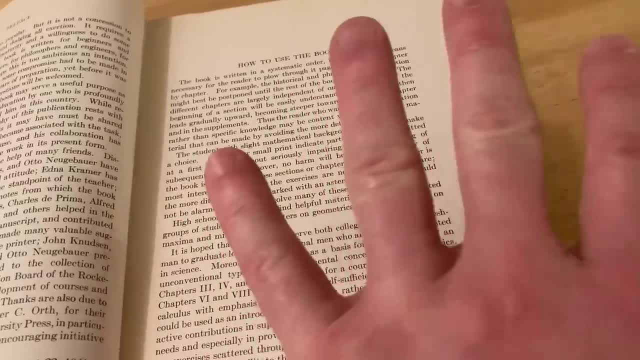 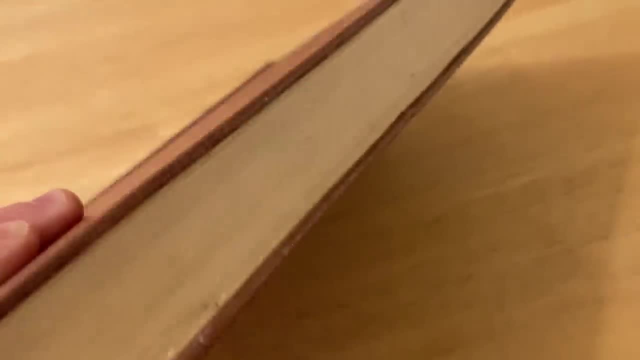 various sections in this book And he just explains so well And I'm going to show you some of the really cool stuff that I've read in this book. Also, this is a very thick book. I mean, look how thick it is. you can just- I can smell the pages. just a work of art. This is a really 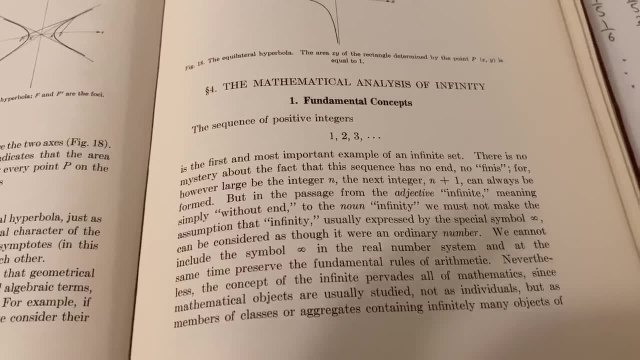 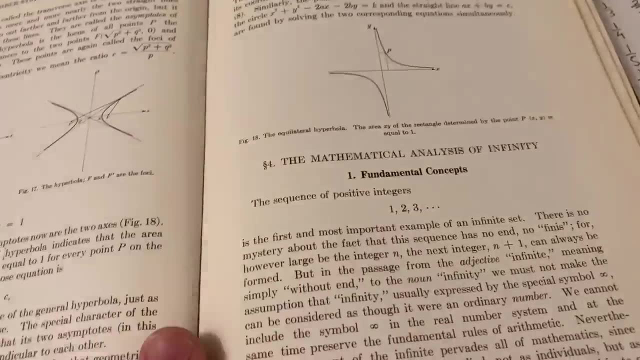 cool section where he talks about the mathematical analysis of infinity. And so basically how I use this book is I just basically open it up And whatever page it lands on, I read a little bit. So a few days ago I was laying in bed and I opened this book up and I landed on this page. 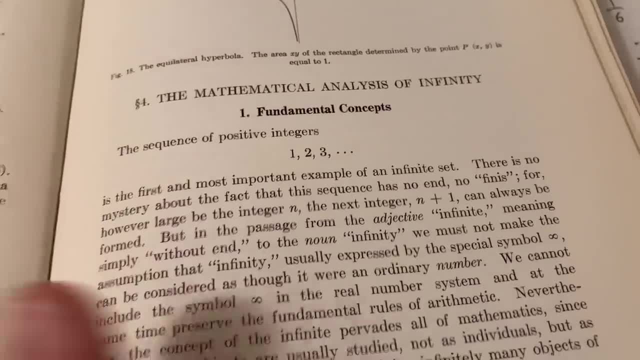 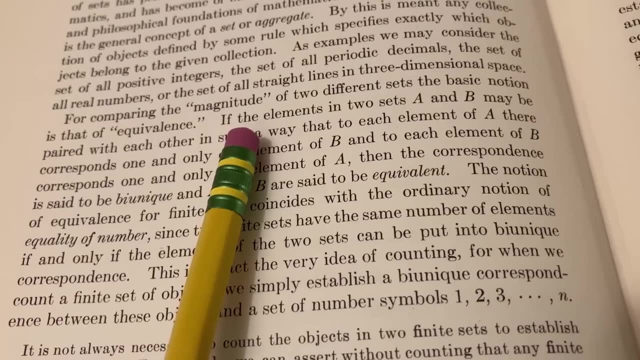 So this is really cool And this is extremely well written. I've never seen a more clear explanation of infinity than in this book here Here Courant talks about what it means for two sets to be equivalent. He says if the elements in two sets, A and B, may be paired with each other. 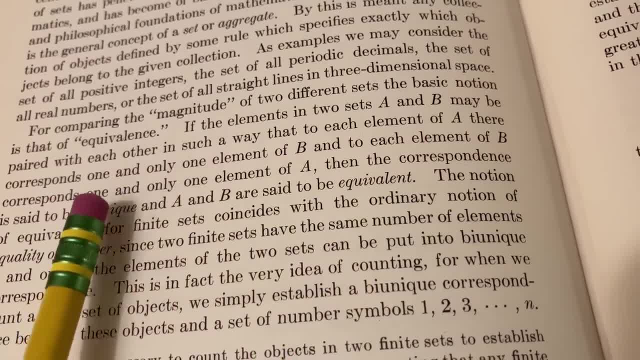 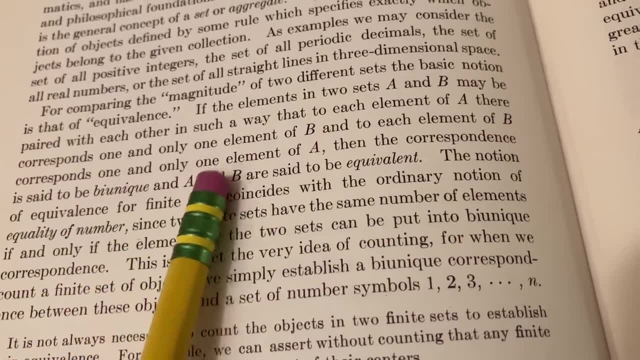 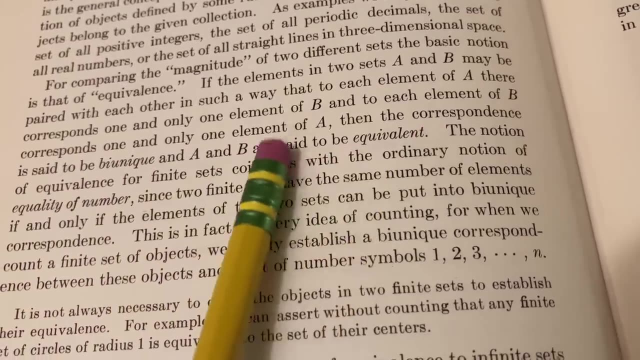 in such a way that to each element of A, there corresponds one and only one element of B, and to each element of B corresponds one and only one element of A, and the correspondence is said to be bi-unique and A and B are said to be equivalent. This is super important, because now 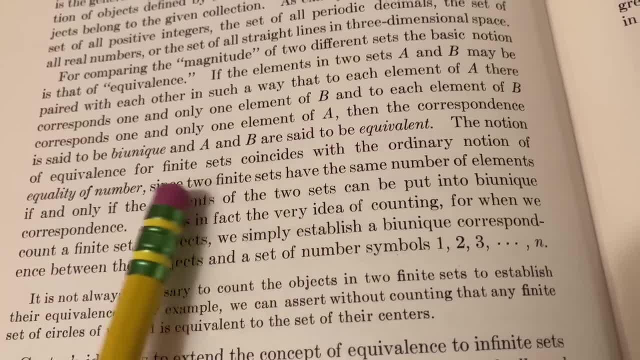 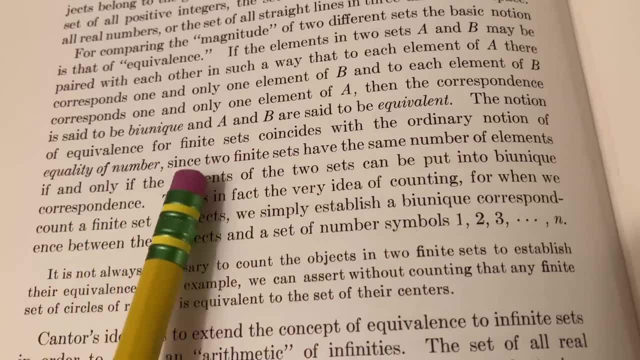 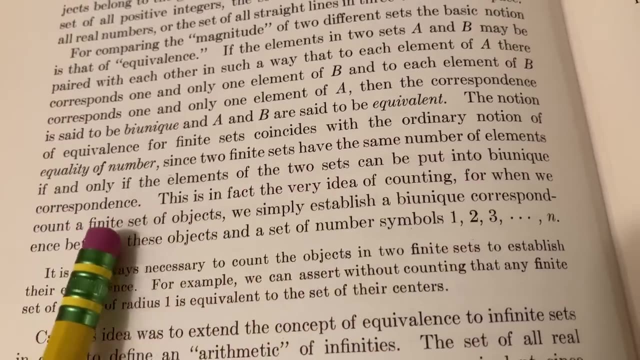 you can compare two sets and you can determine if they're equivalent. And the notion of equivalence for finite sets coincides with the ordering notion of equality of number, Since two finite sets have the same number of elements if, and only if, the elements of the two sets can be put into a bi-unique. 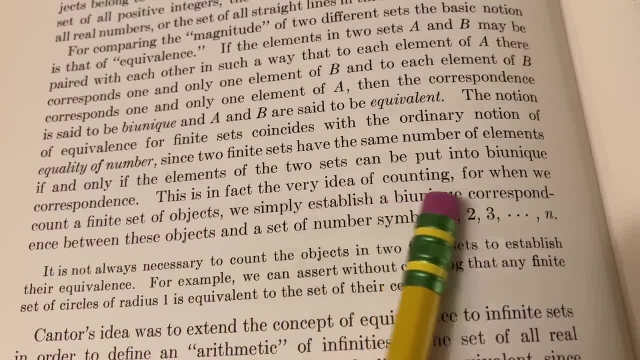 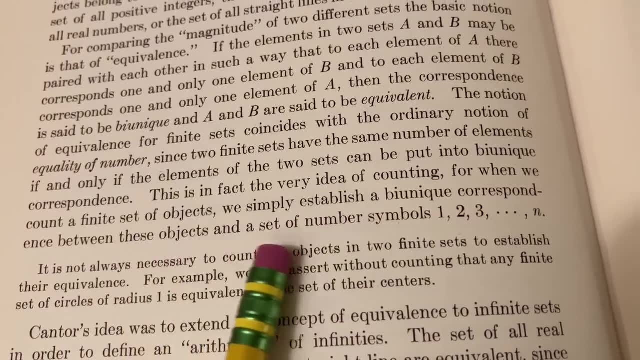 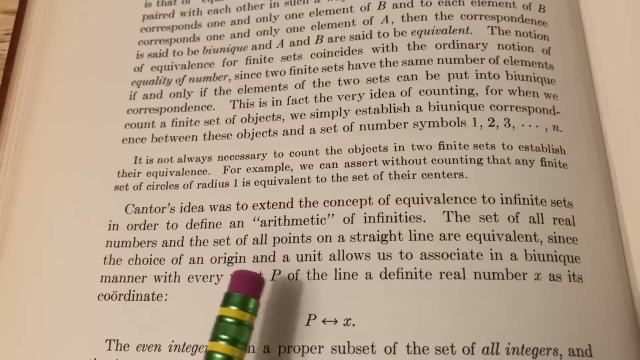 correspondence. He says. this is in fact the very idea of counting, For when we count a finite set of objects, we simply establish a bi-unique correspondence between those objects and the set of number symbols 1 through n. Wow, just incredible. And here he goes on to talk about. 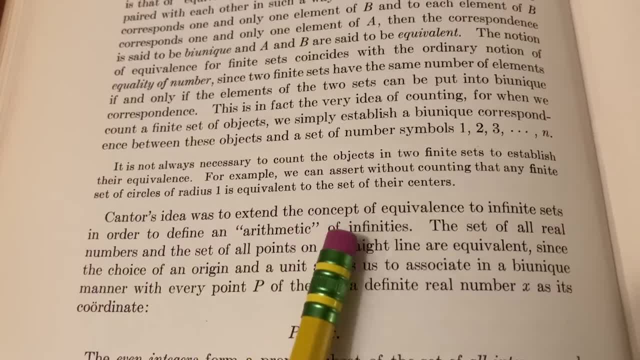 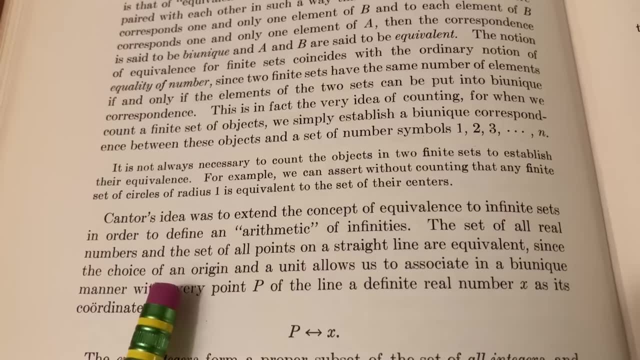 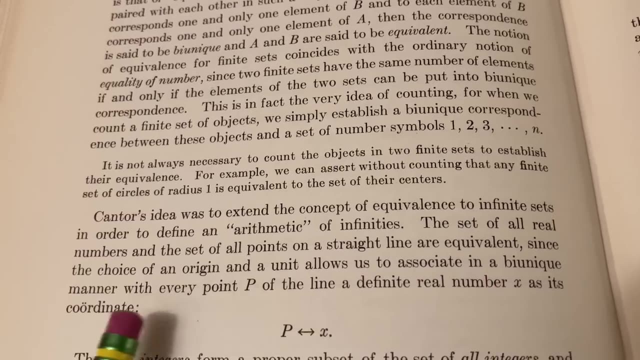 infinites. He says Cantor's idea was to extend the concept of equivalence to infinite sets in order to define an arithmetic of infinities. the set of all real numbers and the set of all points on a straight line are equivalent, since the choice of an origin and a unit allows us to associate in a bi-unique. 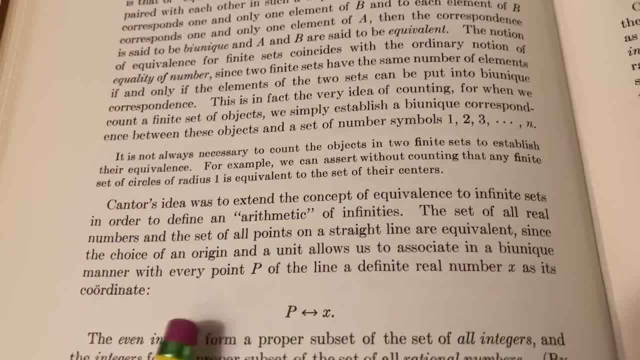 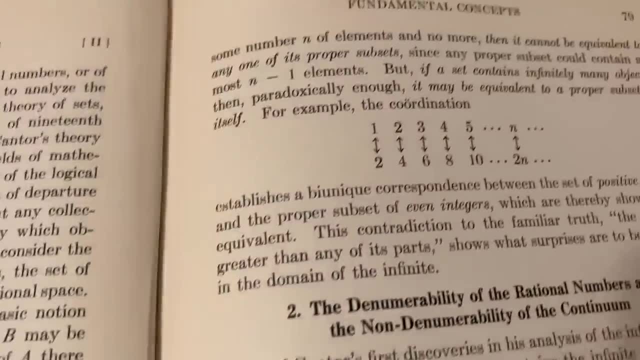 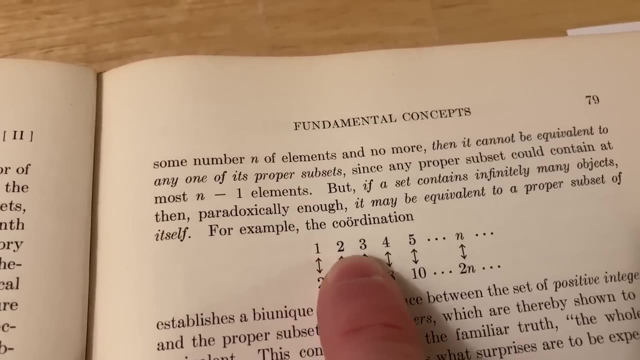 manner, with every point p of the line a definite real number, x, as its coordinate. Then here he talks about the integers and he goes on to show that the set of integers is equivalent to the set of even integers. and you can do that by simply listing the integers 1, 2, 3,, 4, 5 and then to 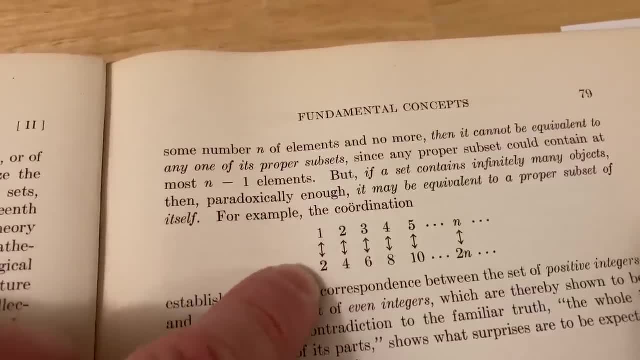 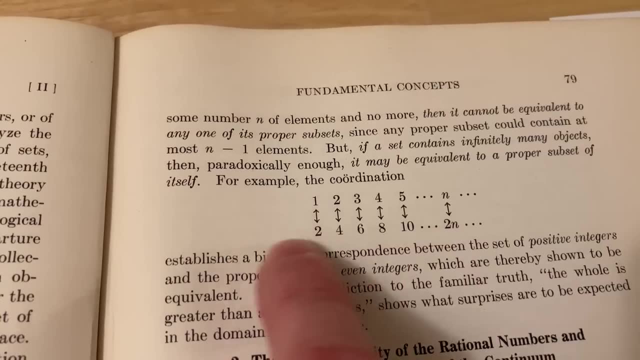 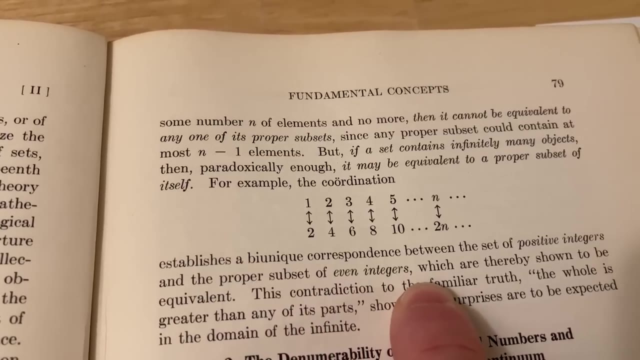 each integer, you assign the following. So for 1, you assign 2, to 2, you assign 4, to 3, you assign 6, basically, you just double each integer and you see, you have this bi-unique correspondence between the set of positive integers and the proper subset of even integers, which are thereby shown to be. 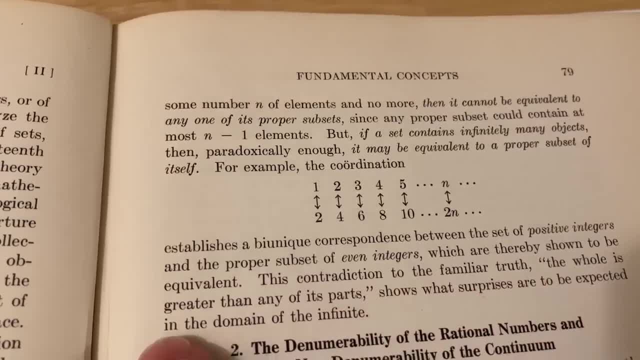 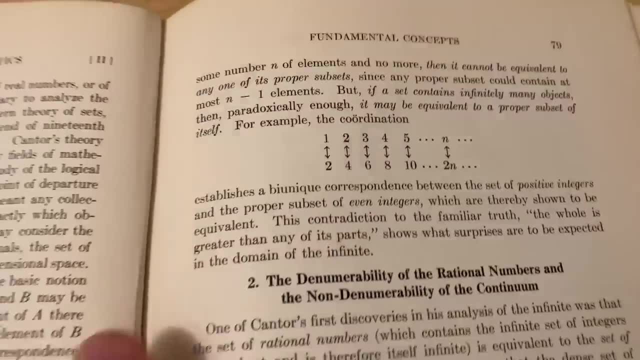 equivalent. This contradicts the familiar truth. the whole is greater than any of its parts. shows what surprises are to be expected in the domain of the infinite. I'm getting goosebumps. This guy, Courant, was amazing. Now for rational numbers. 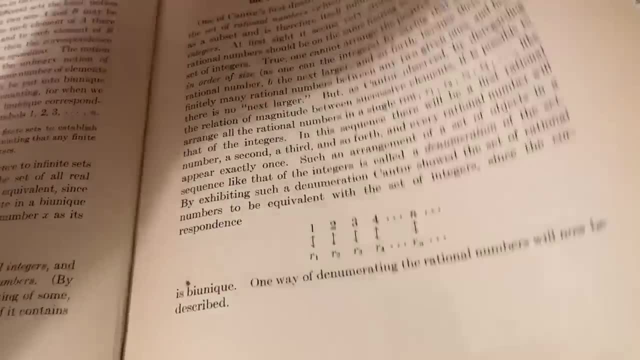 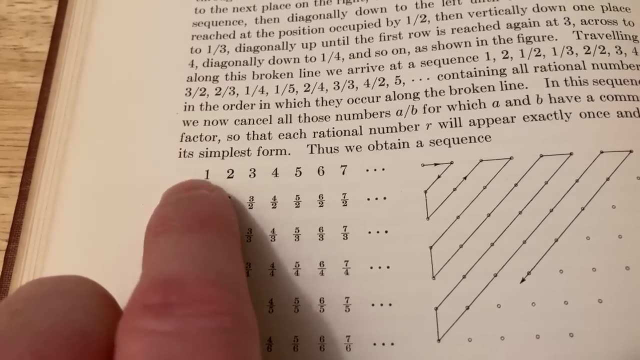 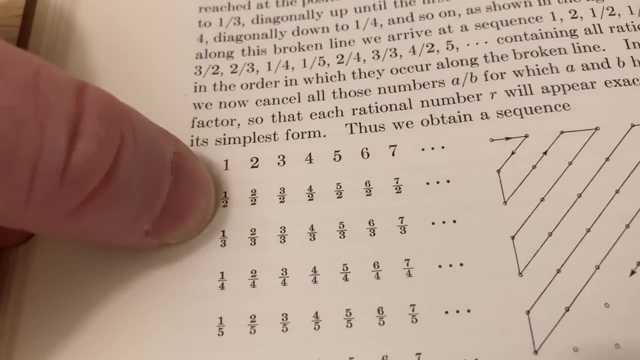 it's not so simple. You can do the same thing, though, with rational numbers, And I think the best way to illustrate that is with this diagram here. So, basically, you list the numbers, all the integers, 1,, 2,, 3,, 4,, 5,, 6, 7.. And then you create this chart. So you take 1, and then you divide it. 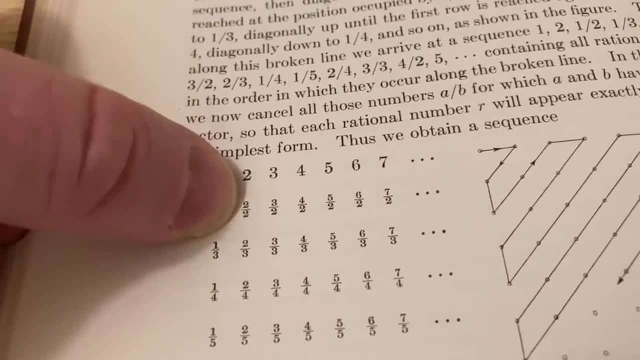 by 2,, by 3,, by 4,, by 5.. Take 2,, divide it by 2,, by 3,, by 4,, by 5, et cetera. Take 3,, divide it by 2,. 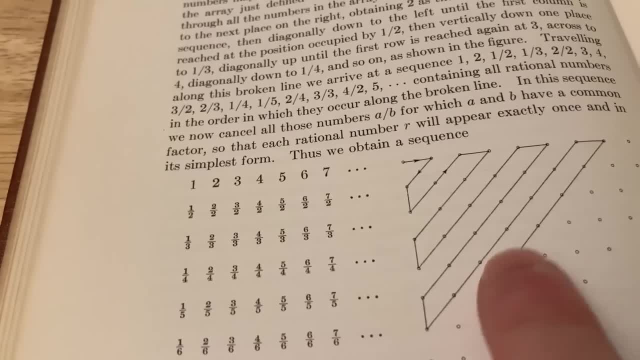 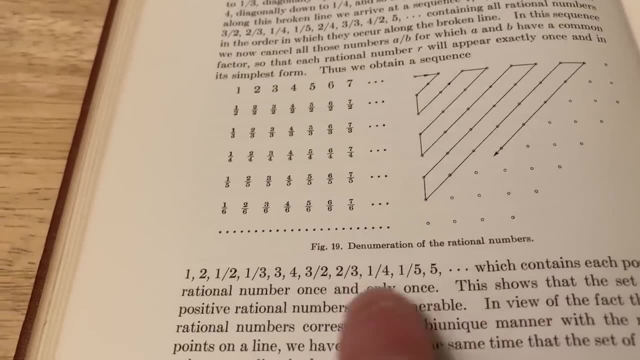 by 3,, by 4,, by 5,, by 6,, et cetera. Do that for each of the integers, And then you can trace out all of the numbers using this system here, And then you basically eliminate duplicates, For 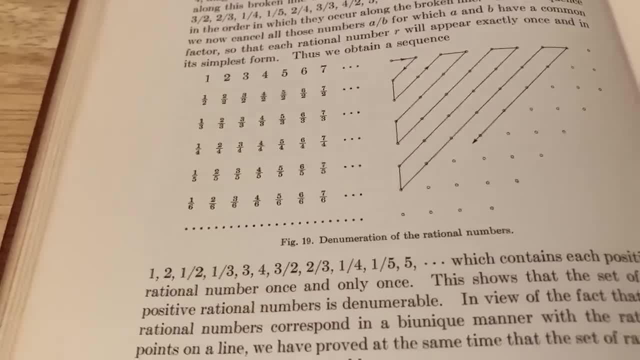 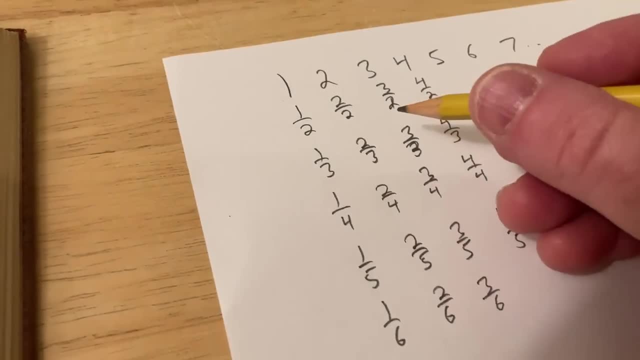 example, if a fraction appears more than once, you eliminate it and only write it once. Let me show you how to actually trace this out. Let me just briefly show you how to actually trace this out. Let me just briefly show you how to actually trace this out. Let me just briefly. 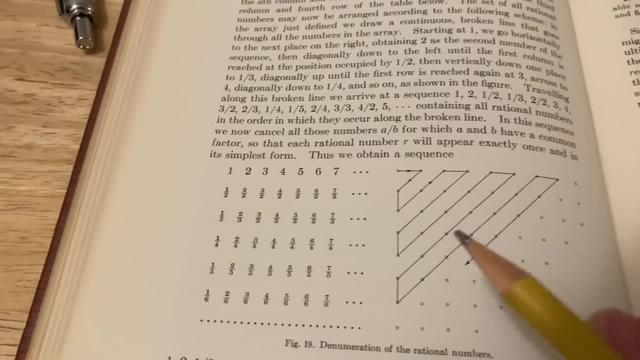 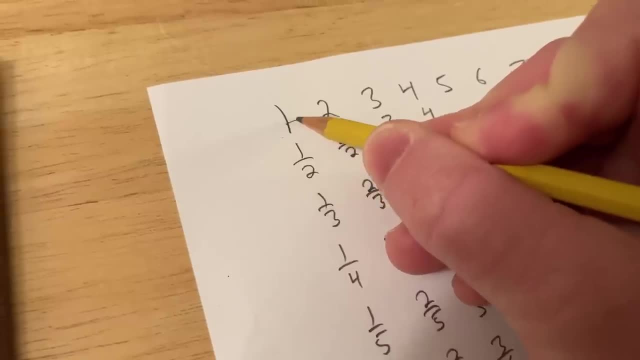 trace this out, Because if you look in the book here you can see the pattern, but you don't actually see it on the numbers. So it's actually pretty simple Basically. you start here at 1, and then you go across like this: Okay, and then you come down, and then you go down 1 like this: 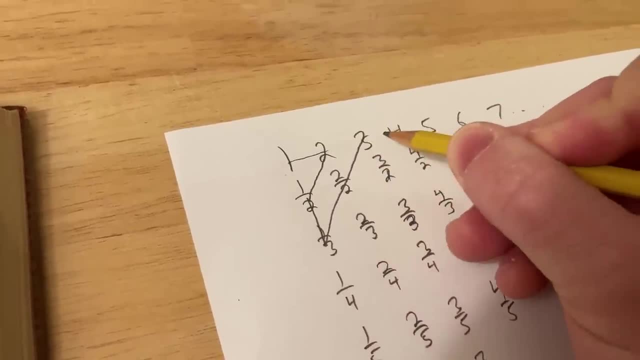 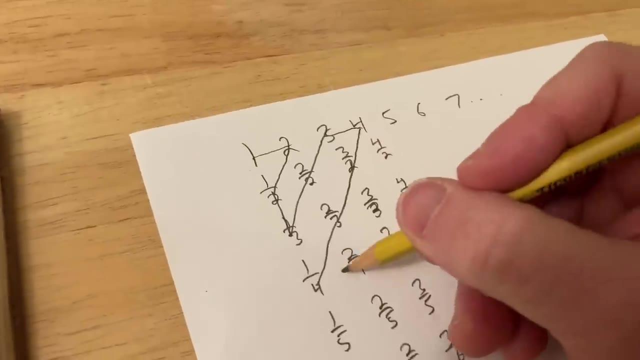 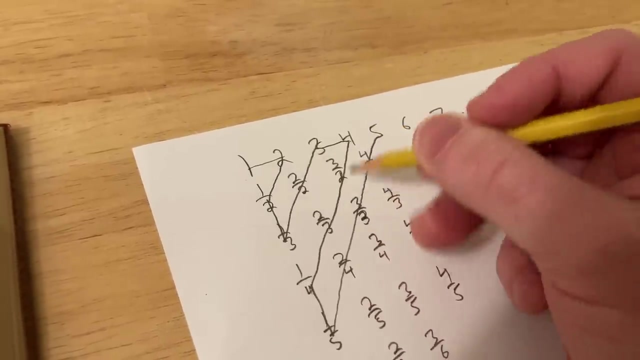 Okay, and then you go back up, Then you go across, Then you go down here, like this, And you see, we're getting every single number in this beautiful chart And then basically you list- okay, you just keep doing this forever And you list them, and then you eliminate duplicates, It's. 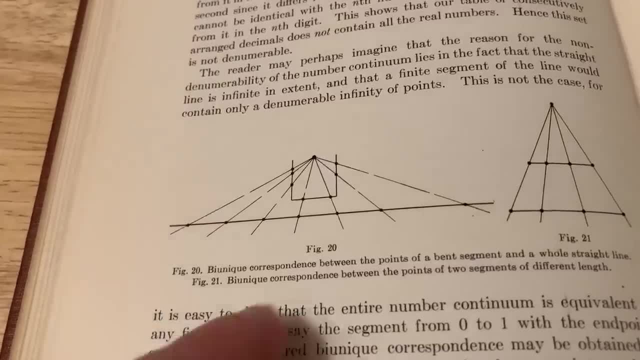 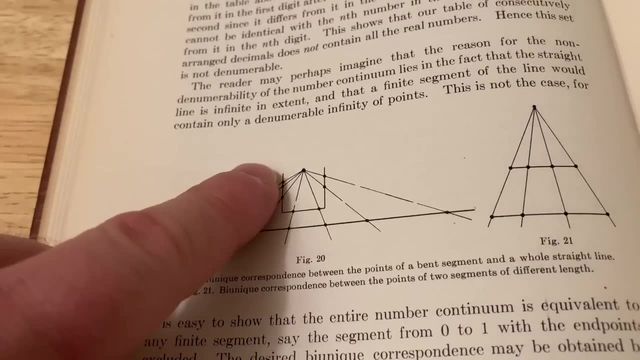 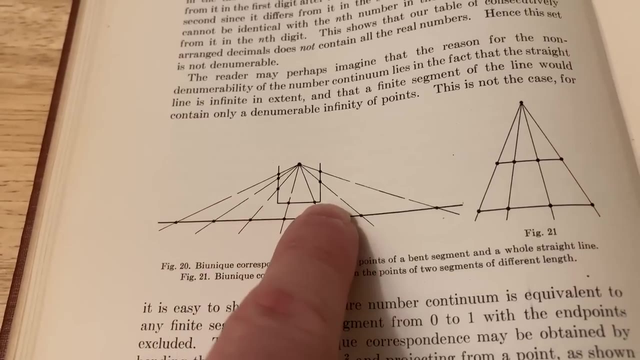 a really beautiful argument. Here's a beautiful diagram that shows that there are just as many real numbers between 0 and 1 as there are real numbers. So Courant talks about how you can take the unit interval, which is this here, and you can bend it at one third and at two thirds And you 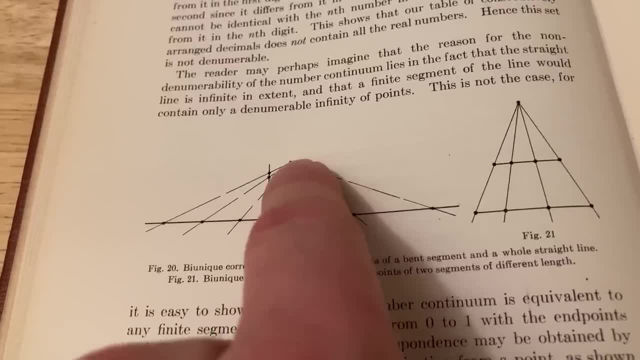 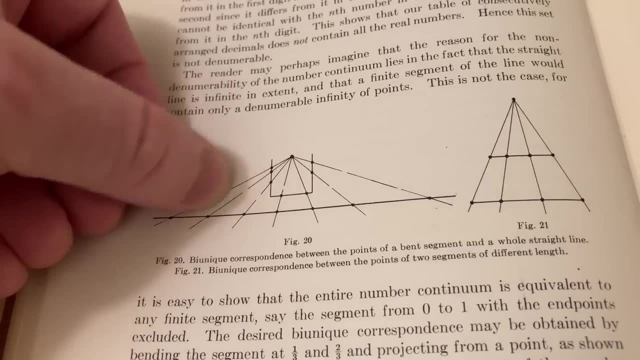 can put a point here and you can just project that point by drawing lines. And you see, if I draw a line here, it touches here and it touches here. So there's a correspondence now between those two points. Do the same thing here. you have a point here and a point here. So you have a. 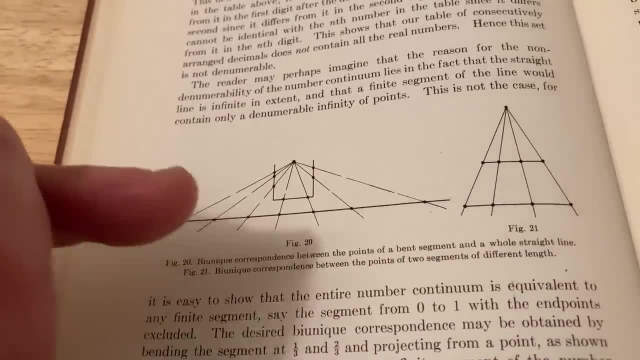 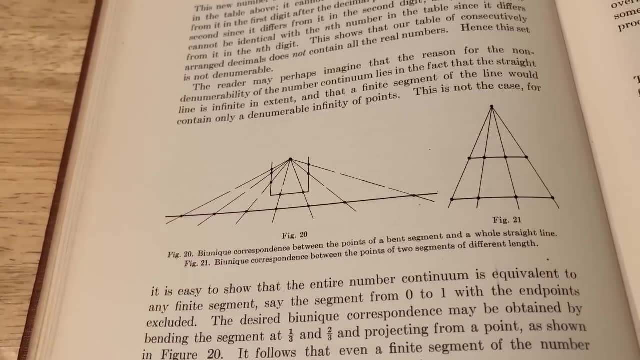 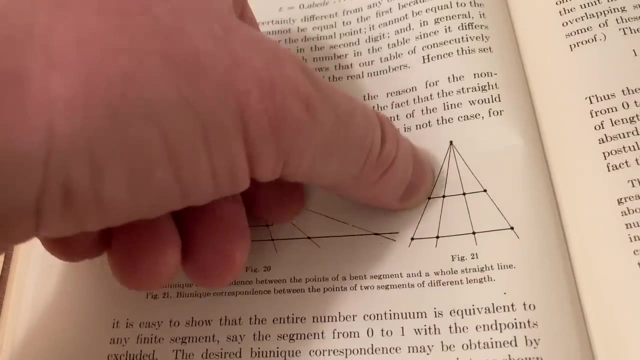 correspondence, a bi unique correspondence between all of the points on the real line And all of the points on the unit interval, And this shows that they are equivalent sets. you does the same thing here with two different line segments By putting a point here and projecting the lines down, so you 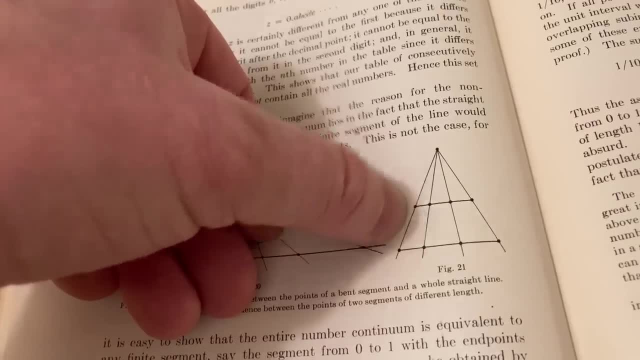 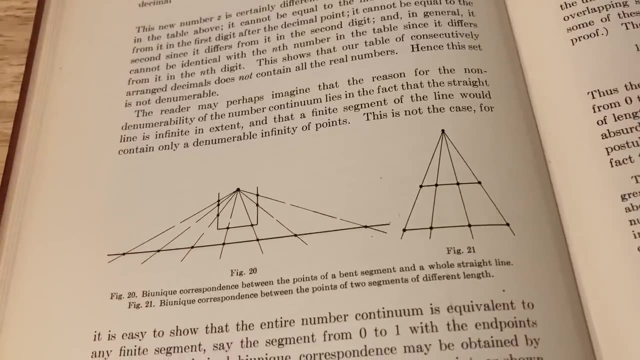 see, this point corresponds to this one and conversely, this one corresponds to this one. so you have a bi-unique correspondence between all of these points. and he does that with just some simple pictures. it's just really beautiful. here he gives a proof by contradiction. it says: let us assume that the 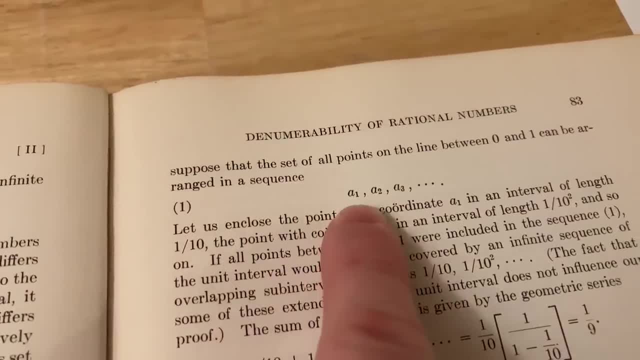 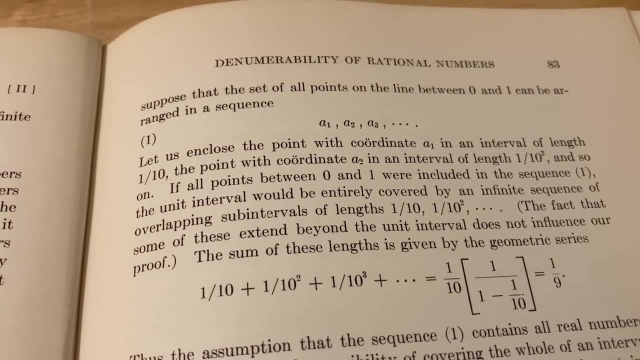 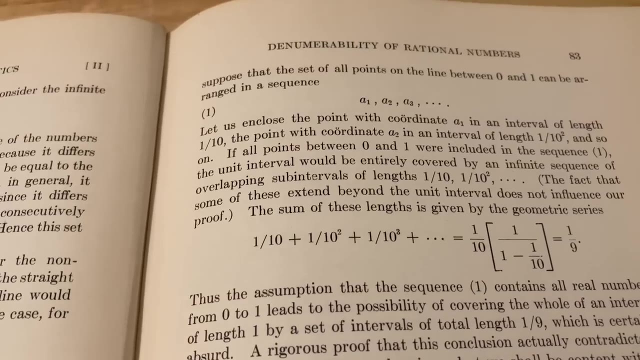 set of all points on the line between zero and one can be arranged in the following sequence: so a1, a2, a3, etc. and what he's going to try to show here is to prove that you can't actually count all of the numbers between zero and one. in other words, the set is not denumerable. so 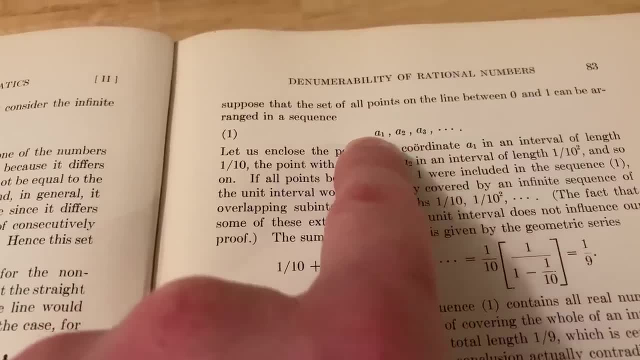 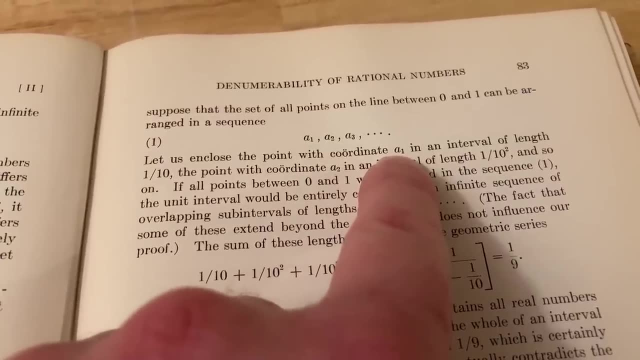 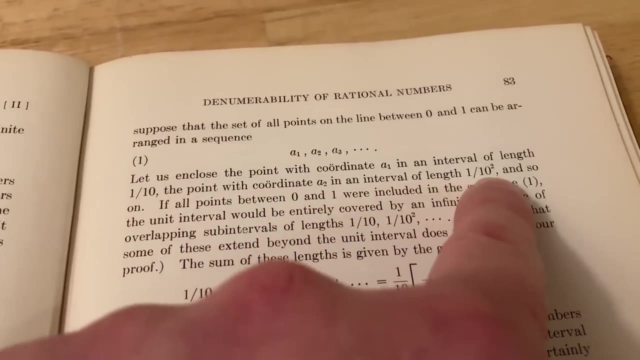 basically suppose it is and you suppose you could just list them all: a1, a2, a3, and then he encloses the point with coordinate a1 in an interval of length 1 over 10 and the point with coordinate a2 in an interval of length 1 over 10, squared, and so on, and then he says: if all of them between zero. 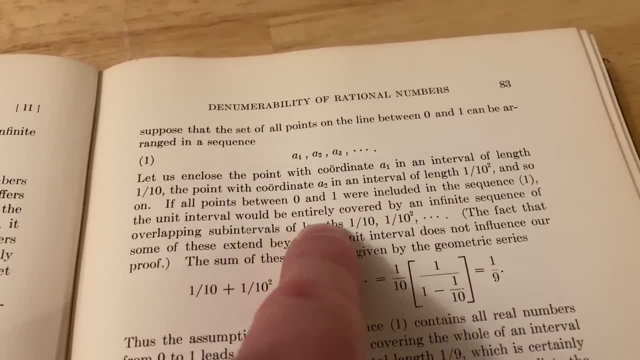 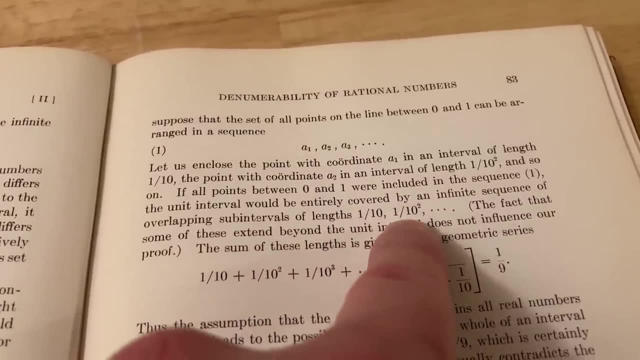 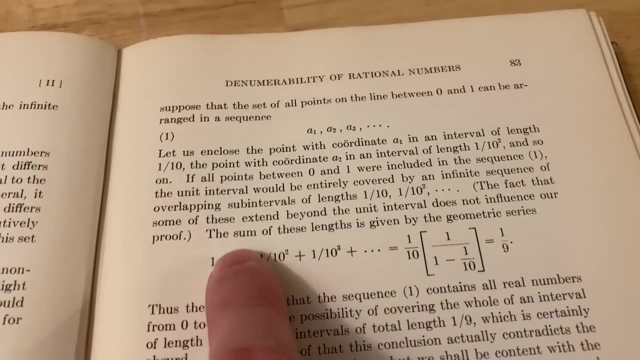 and one were enclosed in this sequence, the unit interval would be entirely covered by an infinite sequence of overlapping subintervals of length: 1 over 10, 1 over 10 squared, 1 over 10 cubed, etc. the fact that some of these extend beyond the unit interval does not influence our proof. and then, if you look at the 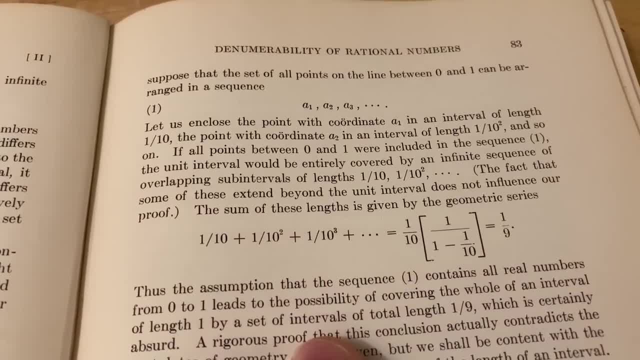 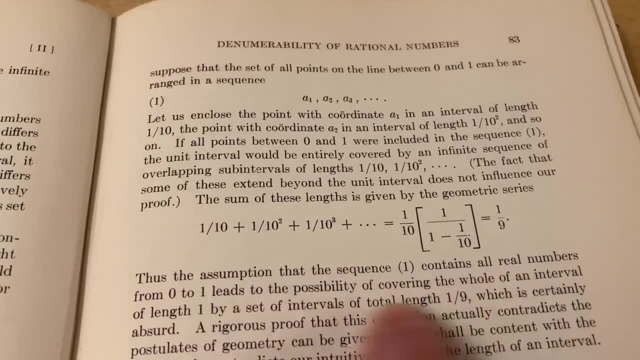 sum of these lengths, you get 1 over 9. and that's impossible, right? because thus the assumption that the sequence contains all real numbers leads to the possibility of covering the whole of an interval of length 1 by a set of intervals of length 1 over 10, and so on, and so on, and so on. 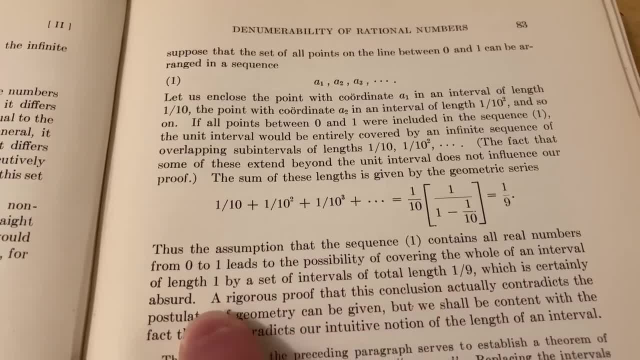 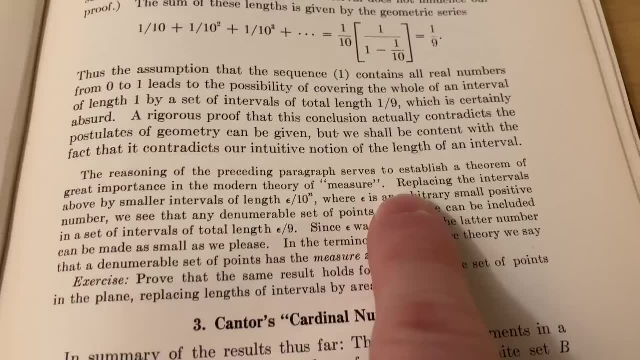 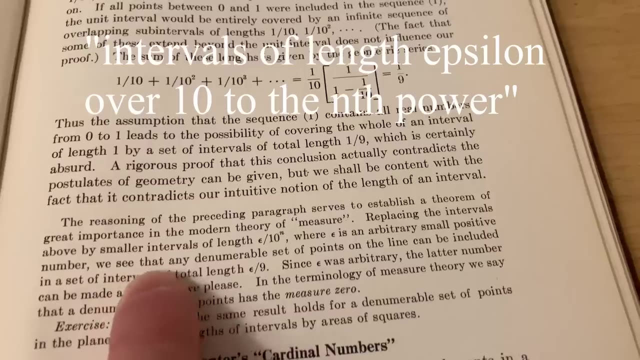 respectively by this Millionen measure of intervals of total length 1 over 9, which is certainly absurd, yeah, just really really beautiful. then here he goes on and talks about how this relates to measure theory, replacing the intervals above by smaller intervals of length, epsilon over 10, where epsilon is an arbitrary small positive number. 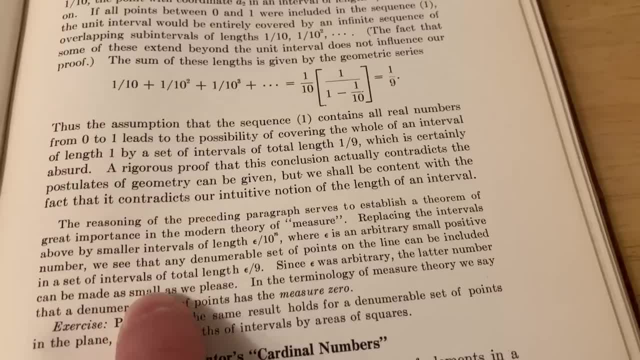 we see that any denumerable set of points on the line can be included in the set of intervals of total length, epsilon over nine, and since epsilon was arbitrary, the latter number can be made as small as we please, writing visual captions just allegedly being the problem. withㄡ Braun School for Substance and 언�ctron in this book. is THAT The Force Of Androgy Gee? You Should Have Seen It. We Are Going to See it Later in thisologia we have aСТ. JUST LIKE This interview. 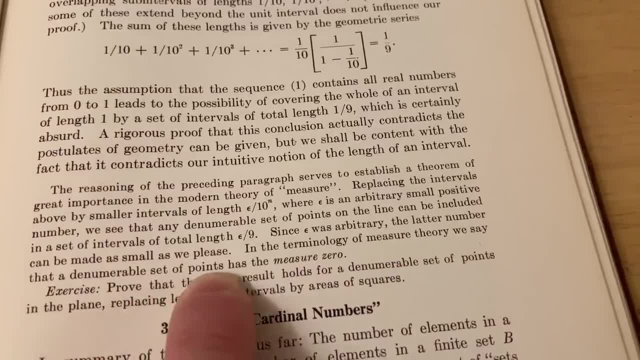 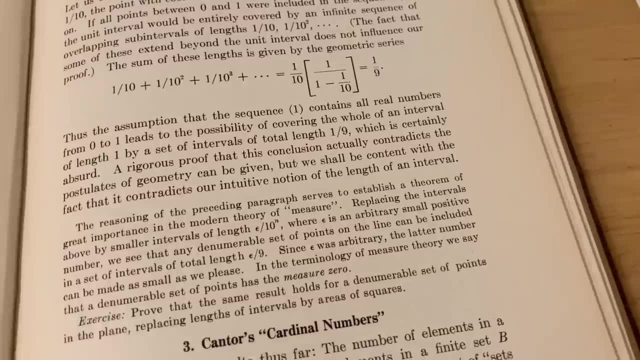 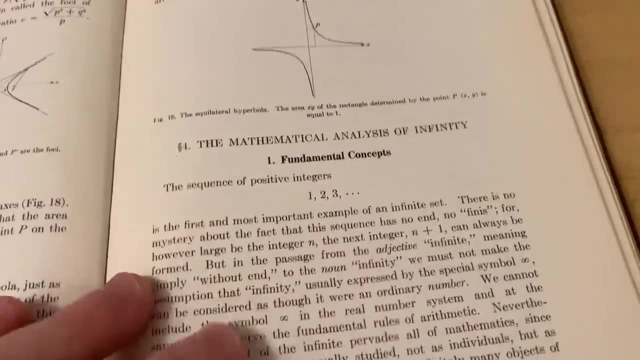 We Love it. In the terminology of measure theory we say that a denumerable set of points has measure zero. So you can prove that using a similar argument here, as he just explained. So I mean he's talking about measure theory only a few pages after introducing, you know, the notion of two sets being equivalent. 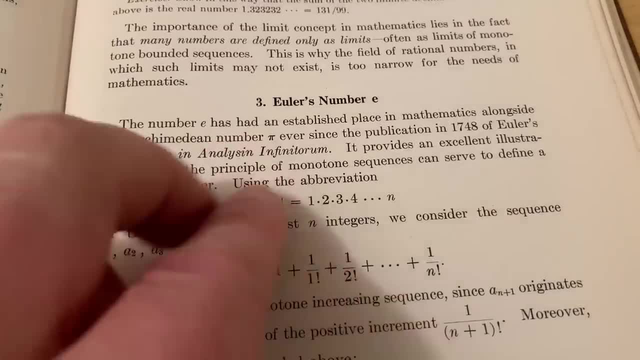 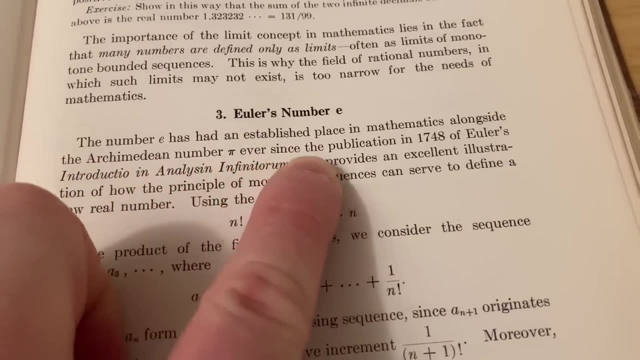 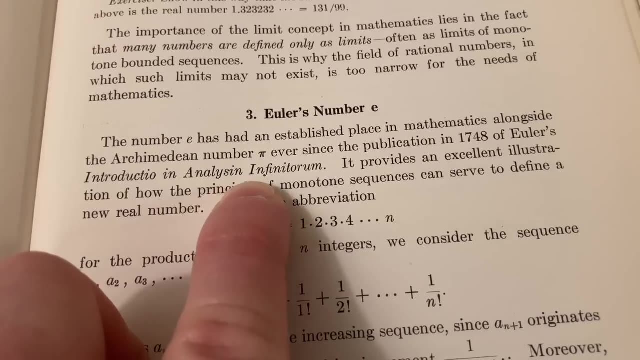 I mean, what a fantastic book. Here he talks about Euler's number e. He talks about how it has had an established place in mathematics alongside the Archimedean number pi ever since the publication in 1748 of Euler's Introductio in Analysin Infinitorum. 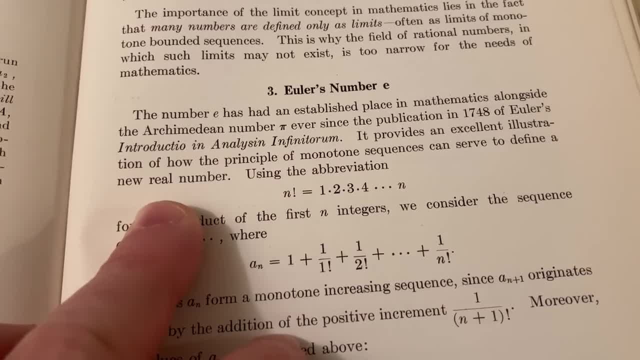 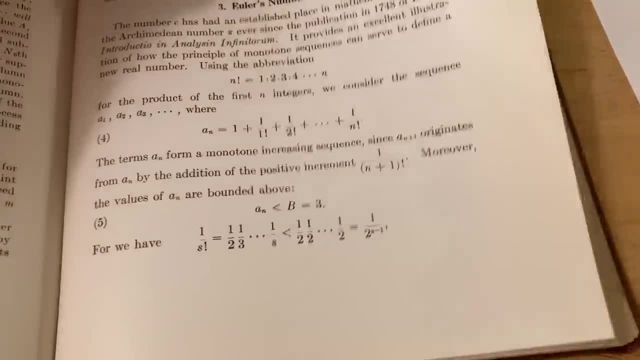 And it provides an excellent illustration of how the principle of monotone sequences can serve to define a new real number. And he goes through it here and defines the number e And then, if you turn the page here, he proves that e is irrational. 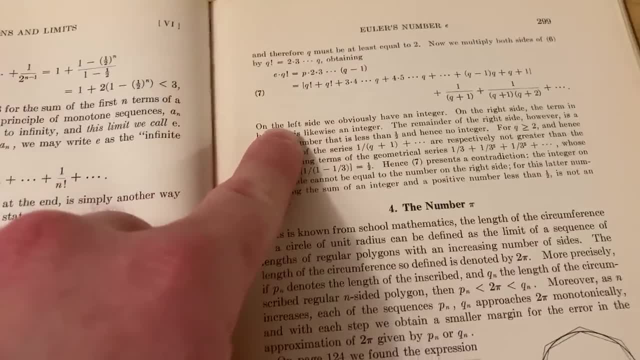 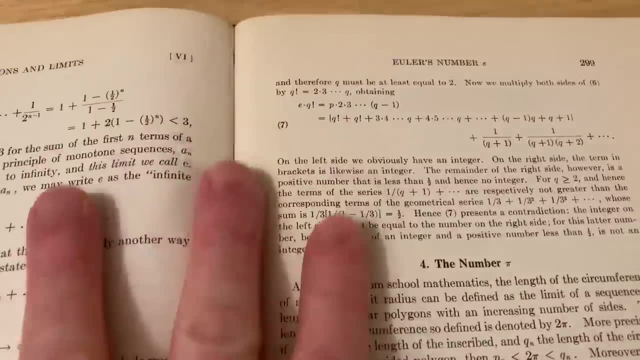 So he gives There's a little proof here showing that it's irrational. And now to understand this proof, you do have to read all of this, because he uses some of the information on this page, But anyone with some math background, I think, could actually understand this. 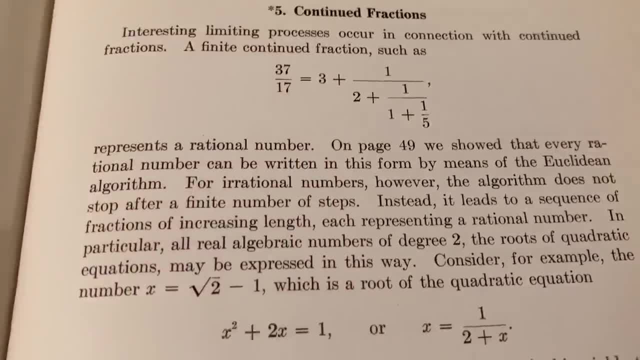 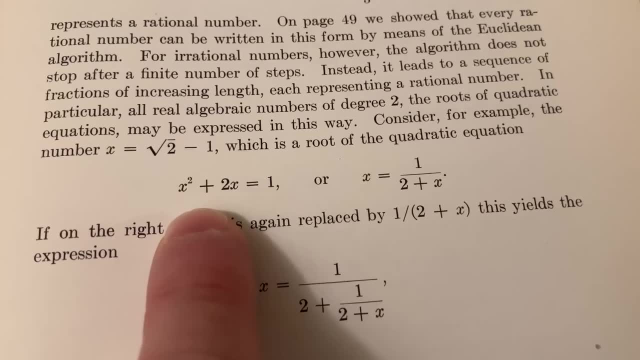 This is a really cool section on continued fractions, And this is really cool. Let me show you. So take this number here: X equals the square root of two minus one, which is apparently a root of this equation. So if you factor out an X here, you'll get X times X plus one. 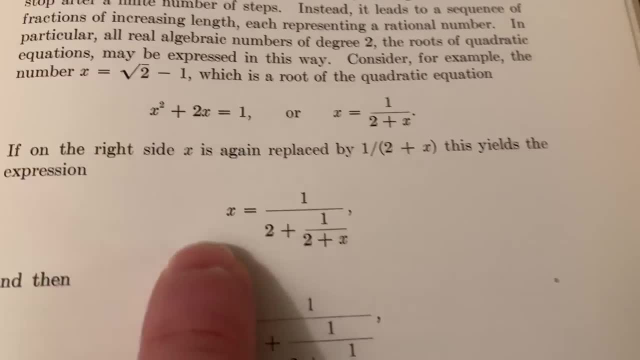 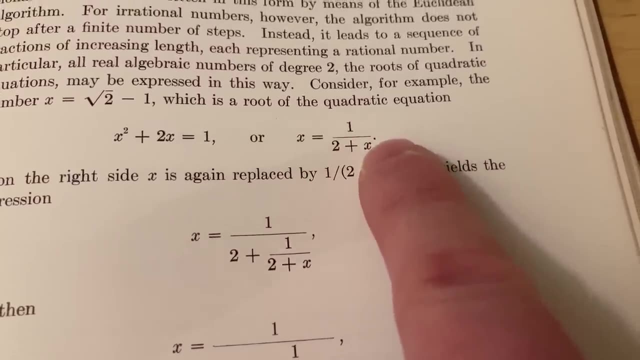 Plus two. You divide by that and you get this. Okay. So now what you do is: you know that X is equal to one over two plus X. So take this X here and replace it with one over two plus X. So you get X equals one over two plus. but what's X? 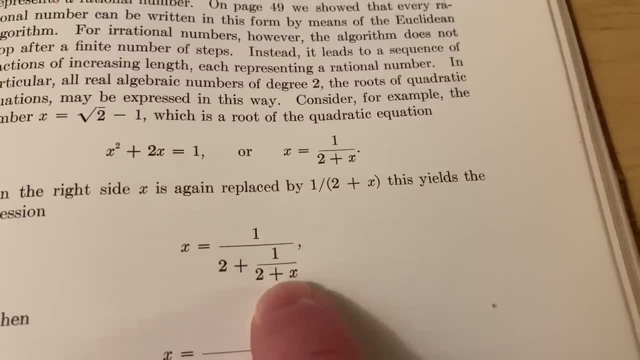 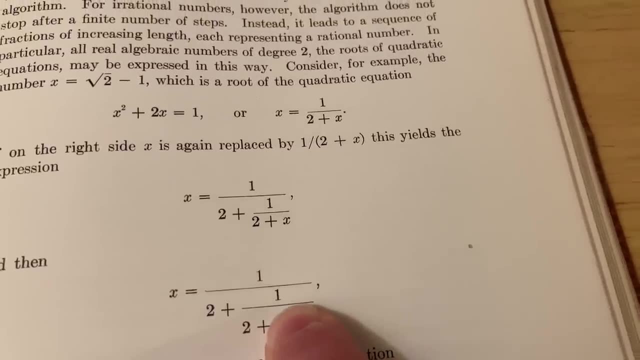 My finger's covering it. Oh, it's one over two plus X, Boom. Then you do it again, My finger's covering it Now. look down here, Boom. You see that. There it is. right, There it is. 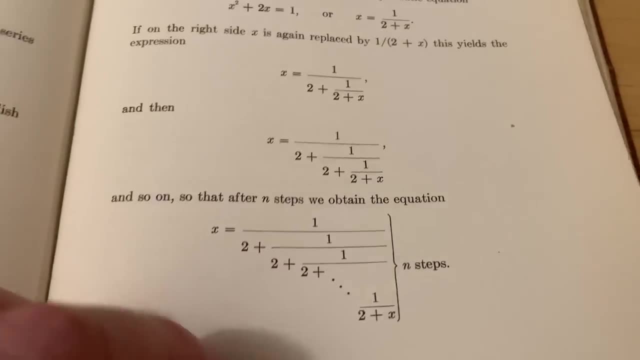 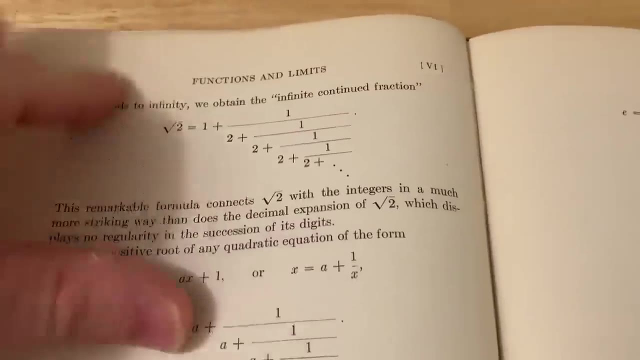 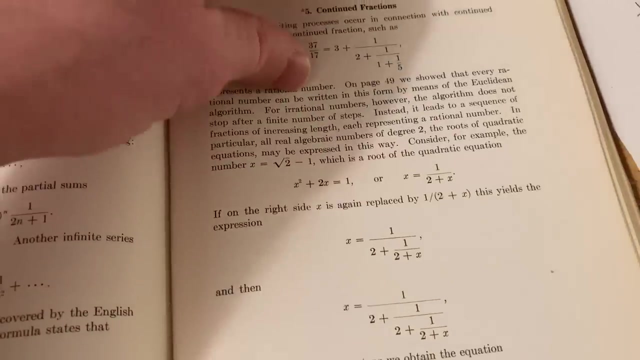 My finger's covering the X. Now it's there, It's forever, And you get, in this case, n steps of this sequence. And then over here, basically, what he's done is he's replaced X with the square root of two minus one and then added one to the other side. 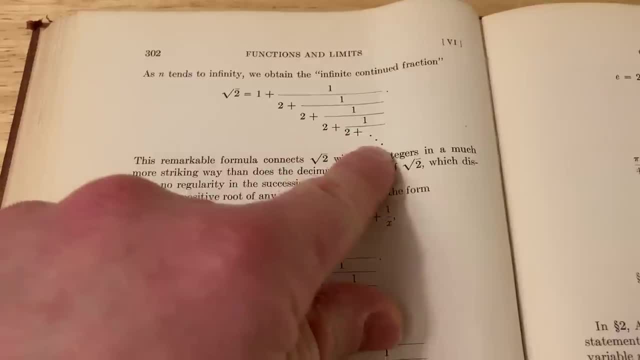 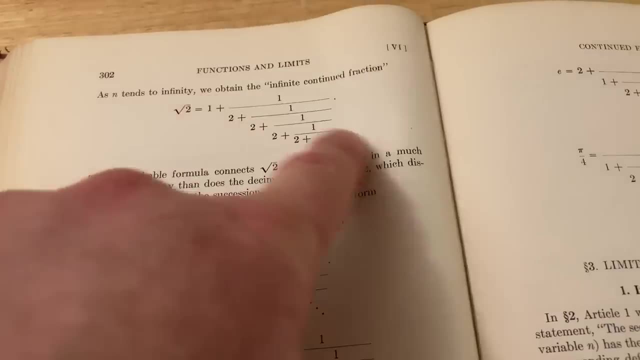 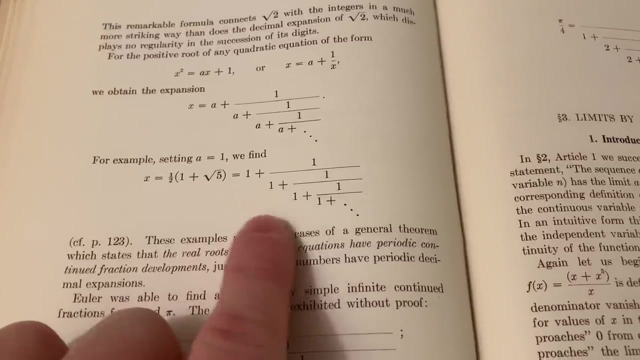 And then he's let: there's the one and you let n go to infinity and you get this infinite continued fraction as he says. Really cool, right, That you can express the square root of two as an infinite continued fraction. And he gives some more examples here of how you can express other numbers as infinite continued fractions. 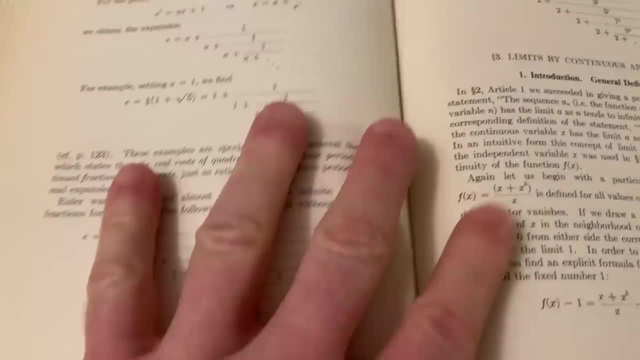 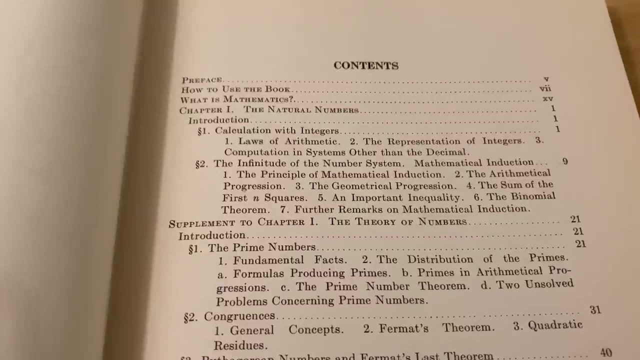 And then here he talks about E. I mean that's really cool, right, And there's a couple other ones here. Just yeah, very, very cool, What an amazing book. So I got a little carried away and I never showed you the contents. 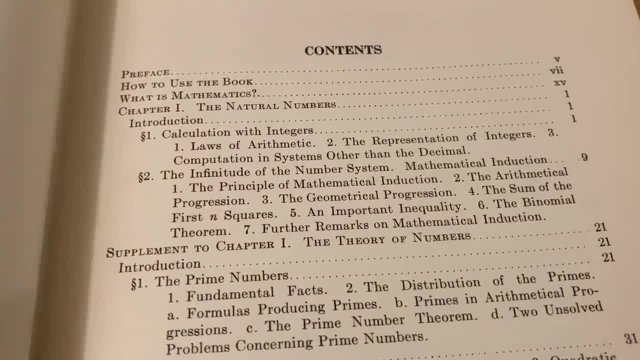 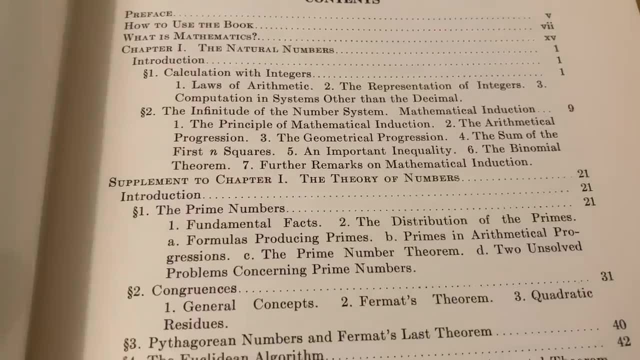 So let's carefully go through the contents so you can actually see what's in this book, because it covers a lot of mathematics. And, I'll be honest, My problem with this book is: I'll pick it up And I'll start reading it and I can't put it down because it's so interesting. 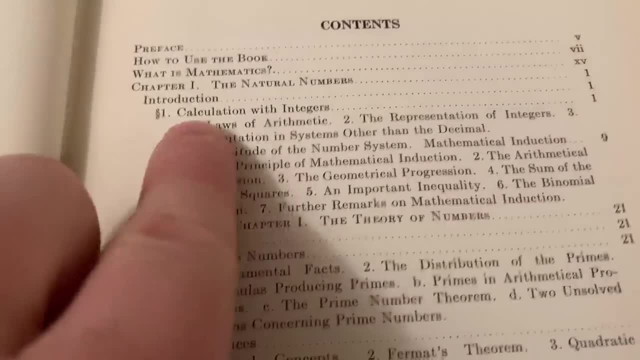 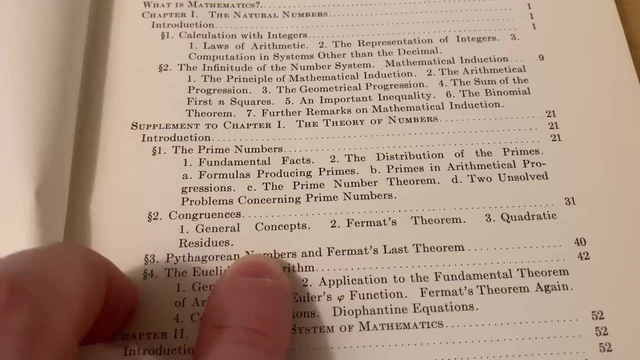 And Courant is such a good writer, So here he talks about the natural numbers. Okay, then a little more on the theory of numbers. All kinds of topics here, all kinds of subtopics and stuff which is really just quite unexpected. 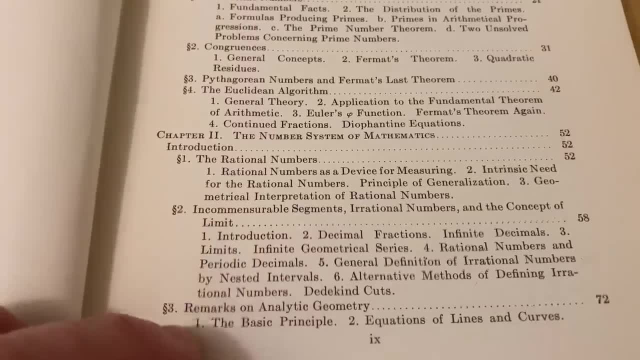 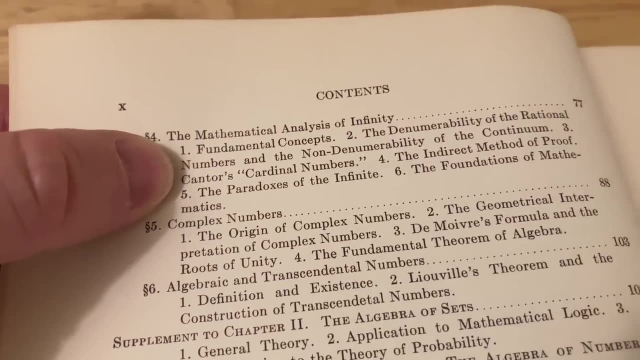 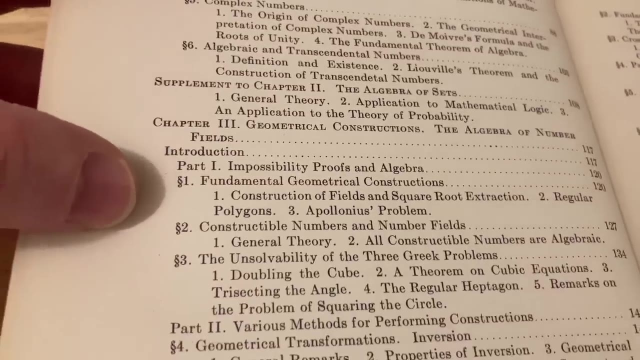 I don't think there's any other book like this. Here he talks about the number system. Let's turn the page. This is that section on the mathematical analysis. Mathematical analysis of infinity Complex numbers, Algebraic and transcendental numbers, Talks about sets. 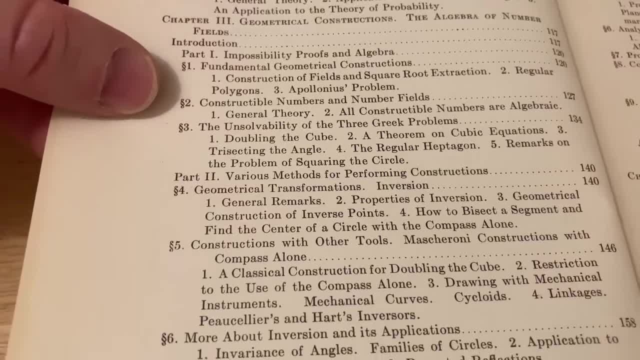 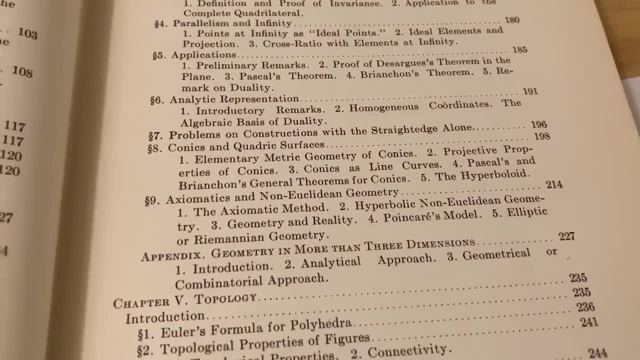 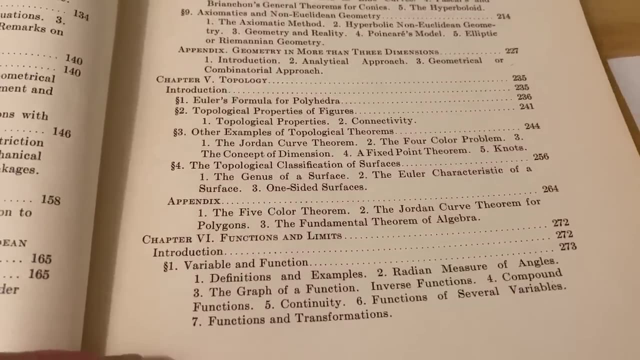 Geometrical constructions- All kinds of topics here. Projective geometry: Here's some more topics here. Just all kinds of things that you wouldn't expect to find. Topology: He talks about topology in this book: Functions and limits. You could actually learn calculus from this book. 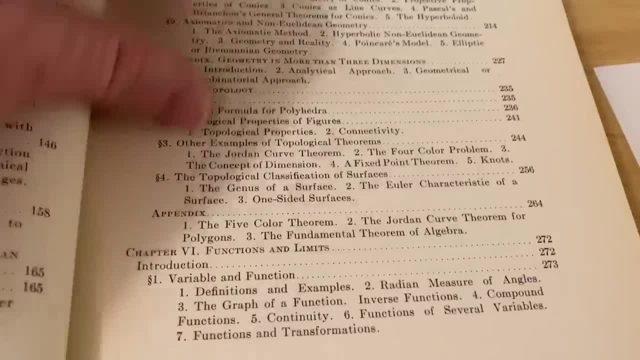 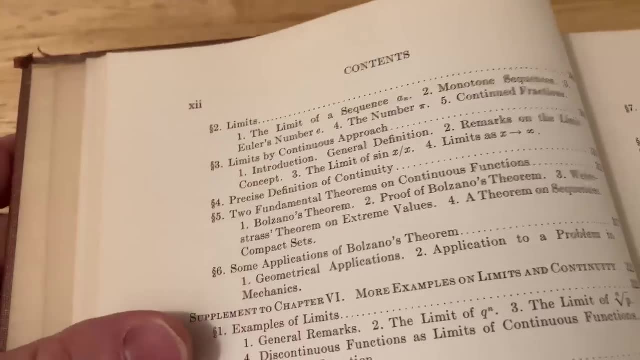 There's enough calculus content in this book- More than enough to actually learn calculus. The only thing that's missing from this book to actually learn calculus with it is the exercises. You would need some exercises for extra practice if you really wanted to learn. 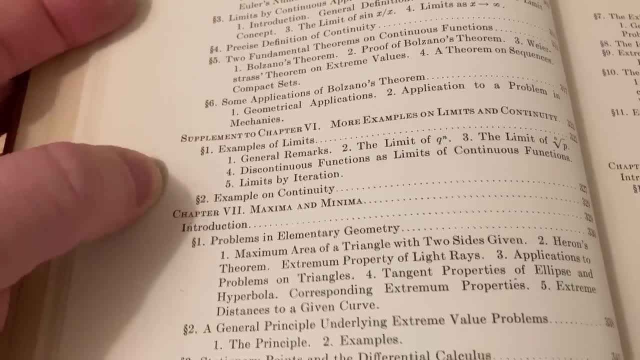 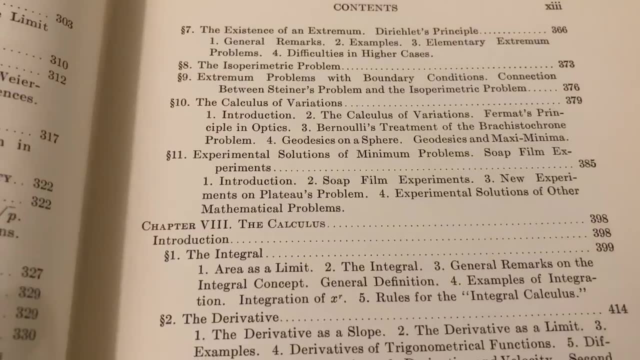 It's enough to offer a full treatment of calculus Maxima and minima, All kinds of topics. Some more topics here. Then here you have, the calculus Talks about the integral, the derivatives, All the things that you would see in a calculus class. 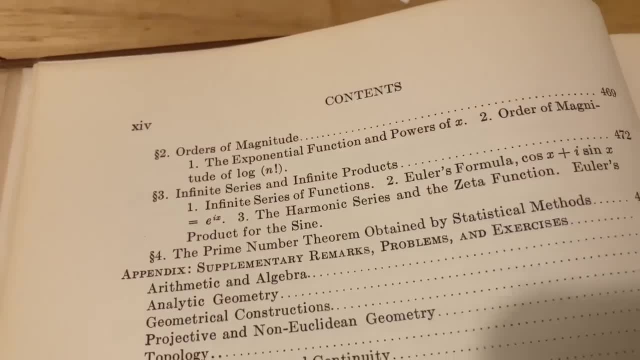 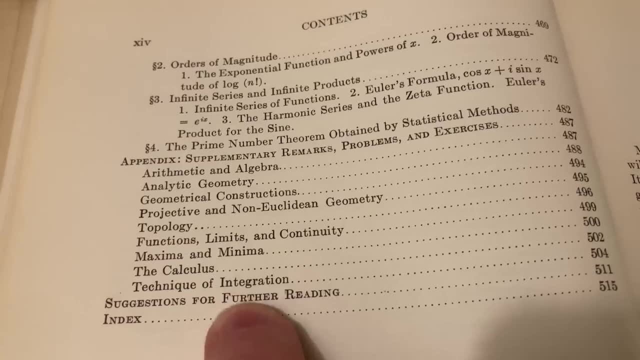 At least a lot of the things you would see. And then here's the last of it: Infinite series and infinite products. Then you've got an appendix with all kinds of things in it- Really cool, Even technique of integration- Cool. Here he talks about topological properties. 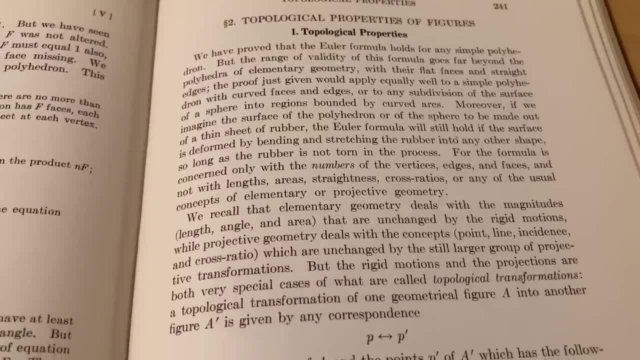 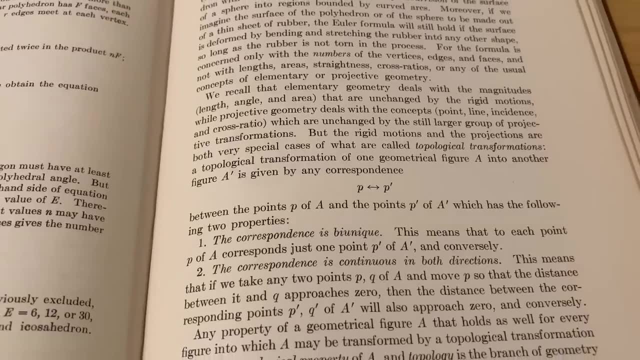 I thought this was really interesting and fairly well written And if you know how to read, you can understand a lot of this. You don't need a lot of math to completely understand it. To understand it completely, you would need some math. 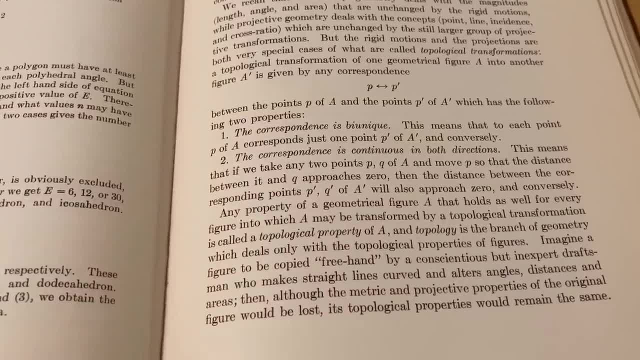 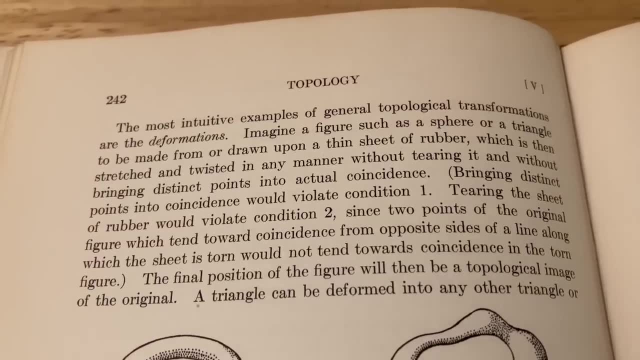 But it's fairly well written in such a way that I think most people could read this and understand most of it. Here Courant talks about topological deformations. It says The most intuitive examples of general topological transformations are the deformations. 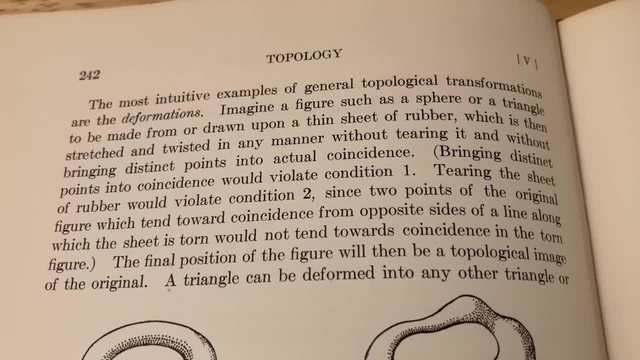 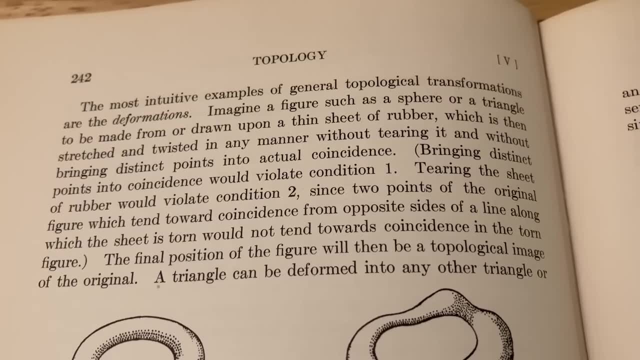 Imagine a figure, such as a sphere or a triangle, to be made from or drawn upon a thin sheet of rubber, which is then stretched and twisted in any manner, without tearing it and without bringing distinct points into actual coincidence. Then here in parentheses, what he's referring to is the stuff. 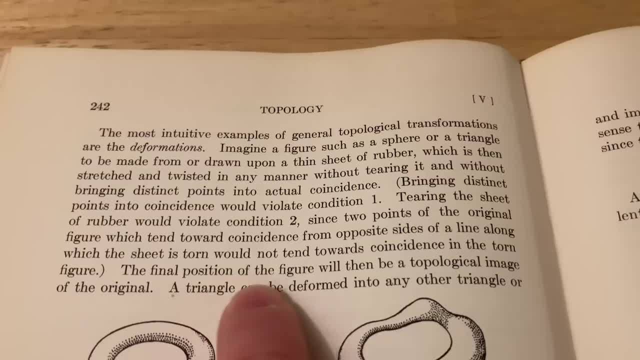 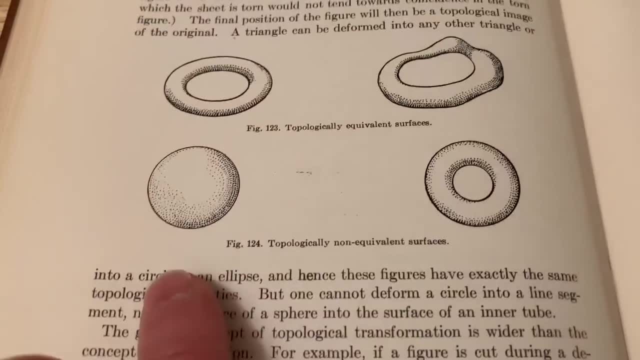 on the previous pages, so I'll skip that. The final position of the figure will then be a topological image of the original. A triangle can be deformed into any other triangle, or into a circle or an ellipse, And hence these figures have exactly the same topological properties. 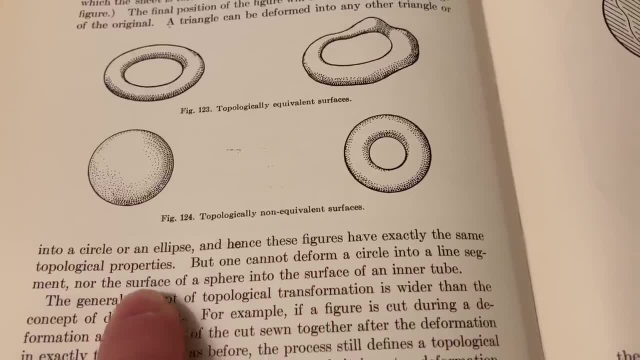 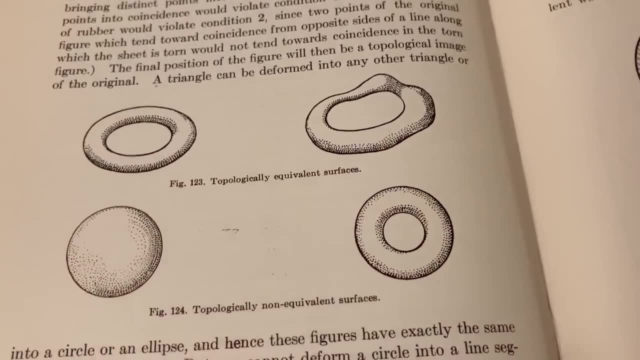 But one cannot deform a circle into a line segment, nor the surface of a sphere into the surface of an inner tube. Here you can see some topologically equivalent surfaces. Really cool And not the kind of thing that you would see at like the beginning of a topology book, right? 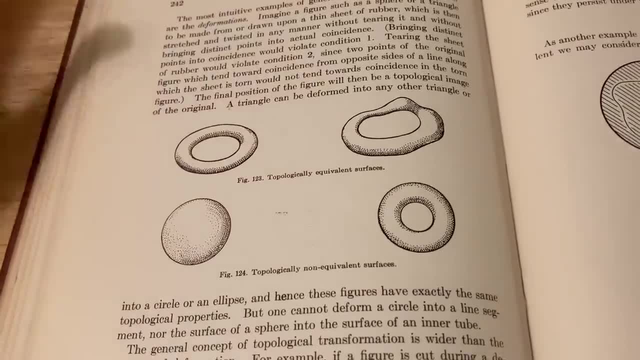 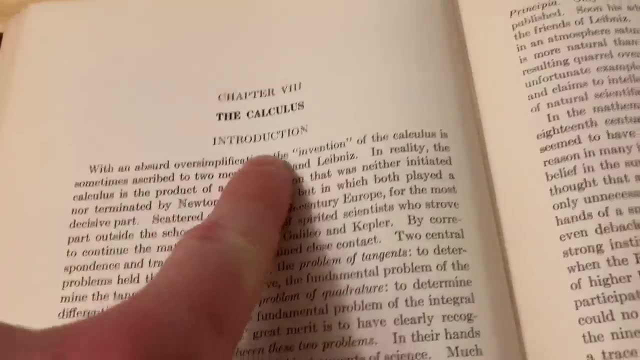 This is something you would learn after you've studied topology for quite some time. Yet you can pick up this book, and Courant talks about it right here. This is the chapter on the calculus. I love how he calls it that Not just calculus, it's the calculus. 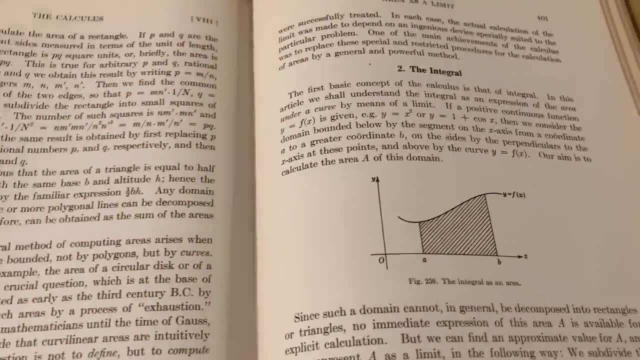 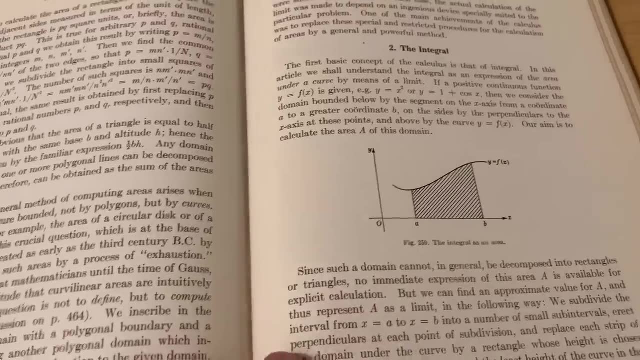 I'm just going to show you some of the stuff in this book. Here you see the integral- Very cool. So it does have basic calculus, but the treatment is very, very different from what you would see in a regular calculus book. The concepts are the same. 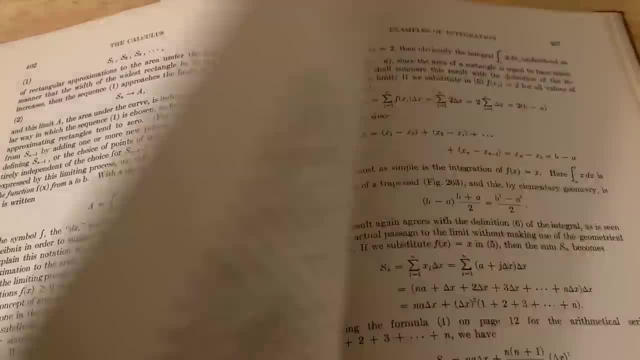 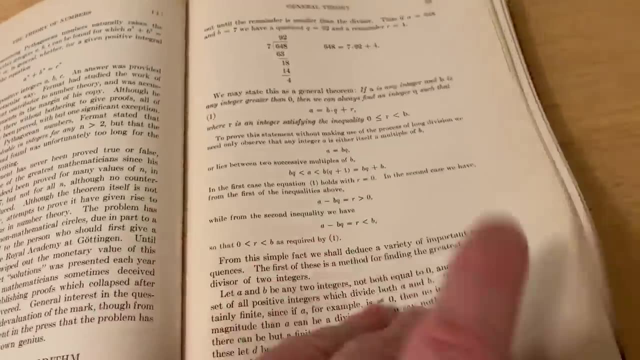 but the exposition, the way it's written, is quite elegant. I think So, as much as I love this book, it is not a perfect book and I think Courant knew that when he wrote it. The big thing that's missing from this book: 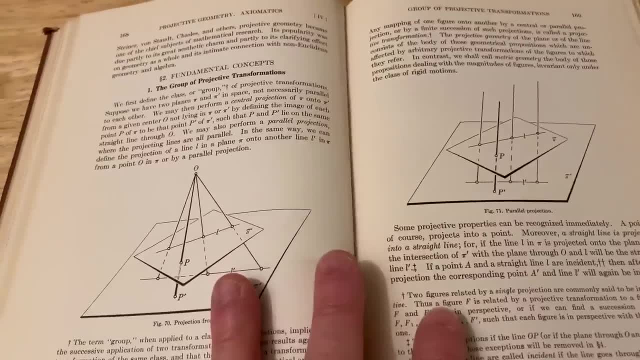 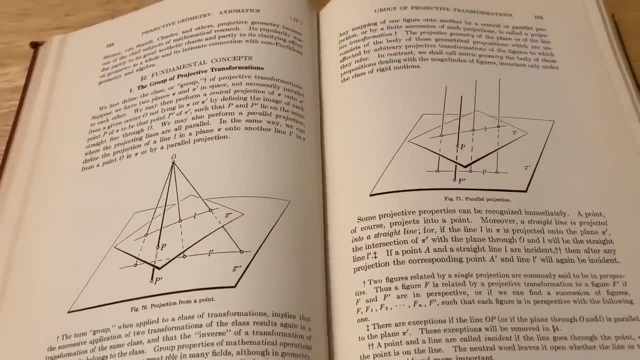 are the exercises. There are some exercises that randomly appear in the book, but they are non-standard exercises and Courant admits that That is not the intention of the book. right, I think that this is a great book for just learning new mathematics. 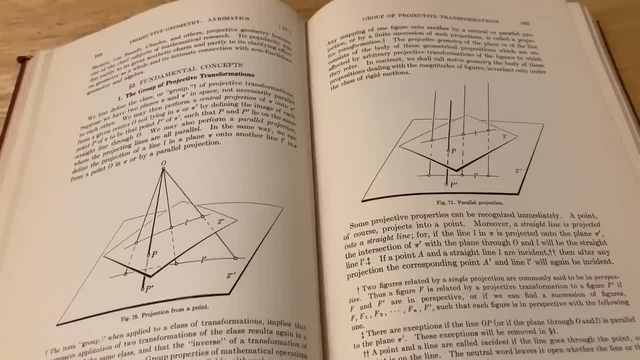 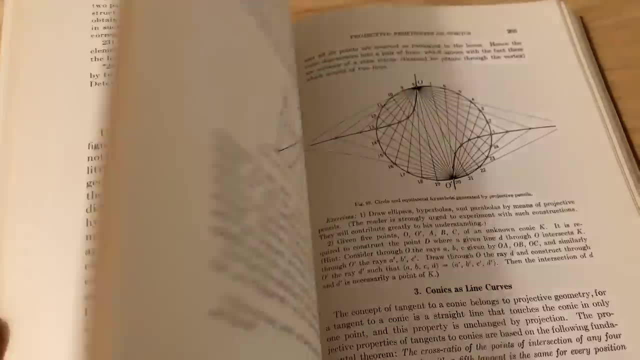 being exposed to mathematics that you haven't seen and revisiting old mathematics in a much more clear way. I feel like Courant explains things a lot better than a lot of other authors. If you look on Wikipedia, he is known for this book. 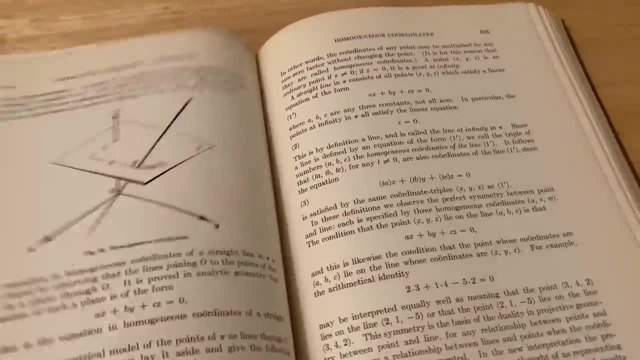 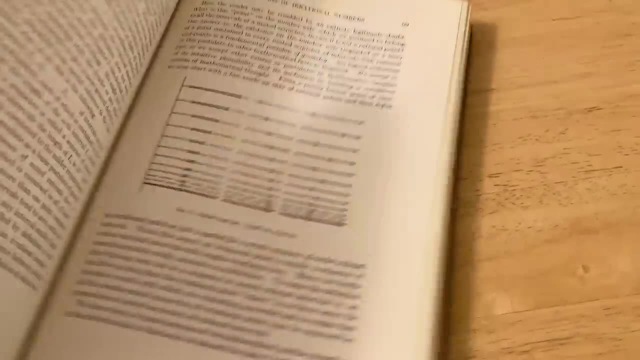 This is a very famous book and, again, the Courant Institute is named after this guy. It's Richard Courant, the German-American mathematician. just brilliant, Yeah, really amazing. Here's a random section on the geometrical interpretation of complex numbers. 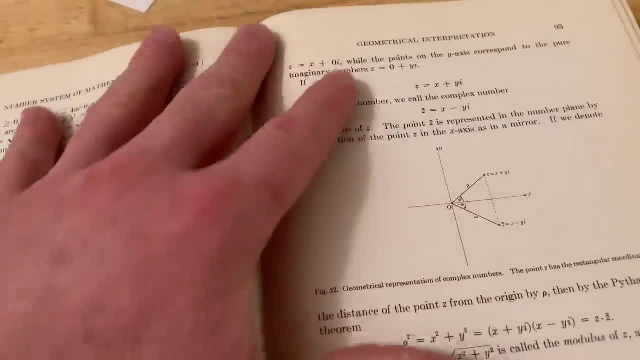 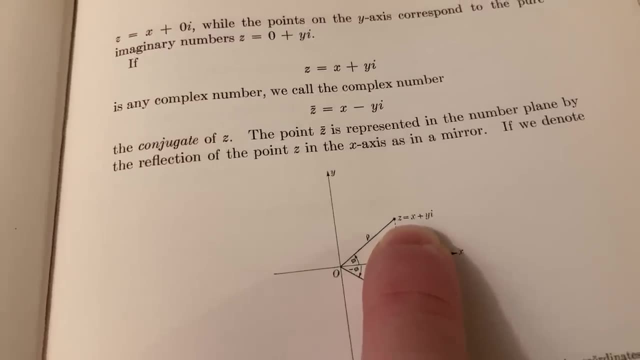 which is also very well written, and I think this is something that most people can pick this up and they can read this and they can understand it. For example, here you see, you have the complex number x plus yi, and then here you have the conjugate. 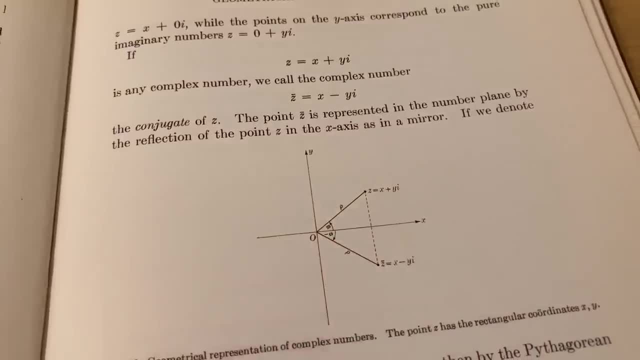 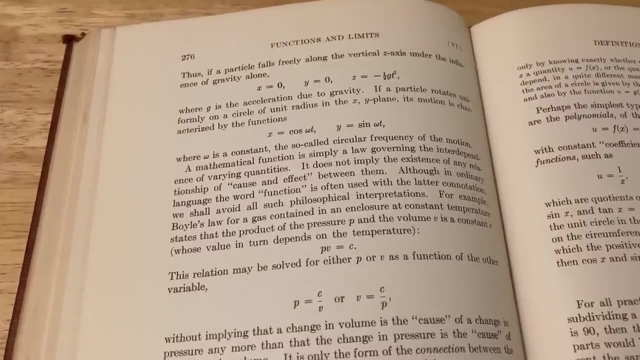 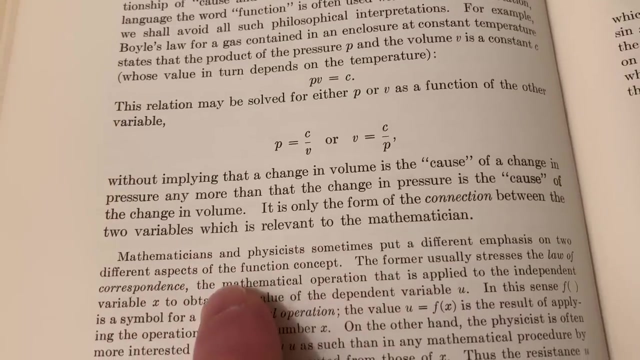 x minus yi. So you see geometrically how they are represented. It's like a mirror image across the x-axis. This is the section on functions and limits, and here he talks about how mathematicians and physicists sometimes put a different emphasis on the two different aspects. 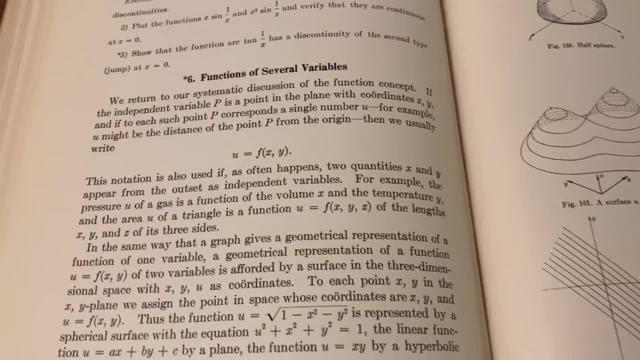 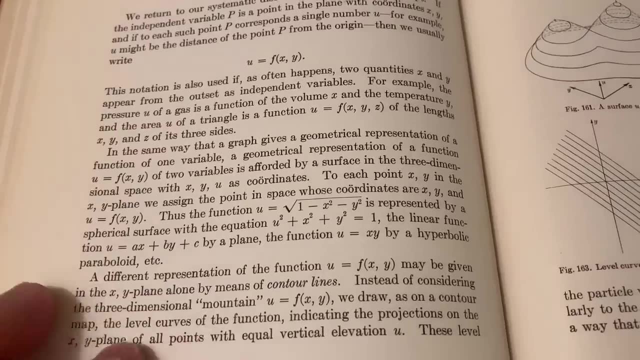 of the function concept and he goes on to explain it quite well. Here he talks about functions of several variables and he talks about how to think of them graphically and he discusses level curves and you can see there's some diagrams here. 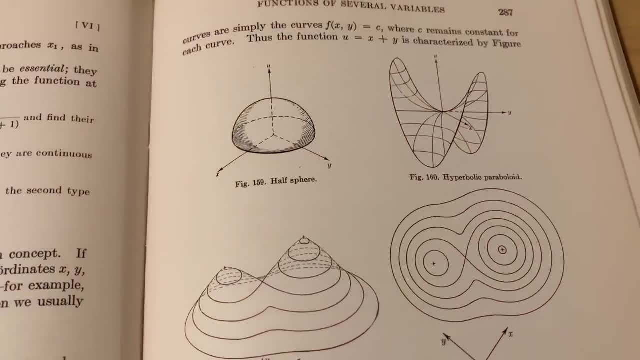 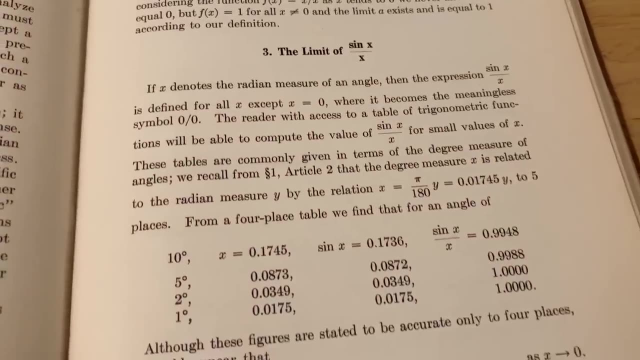 and this is pretty cool- I mean for a book from 1941, I think this is fantastic. Here he has a section on the limit of sine x over x as x approaches zero, and he gives some computations here and then he gives a rigorous proof. 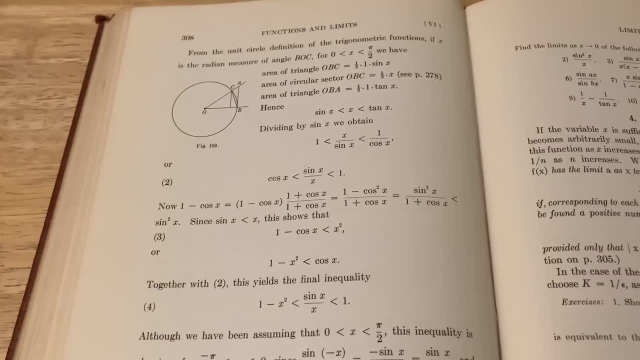 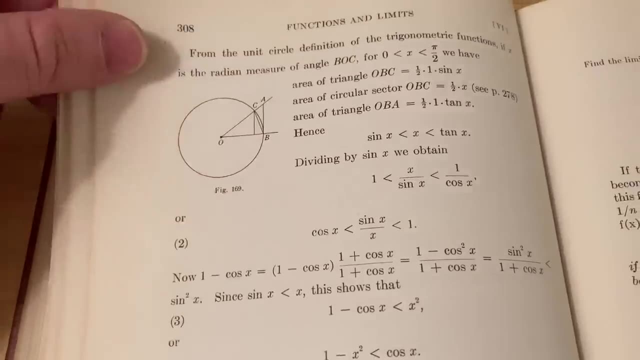 geometrically of the statement here. so it's kind of nice You learn this in a Calc 1 course, and this is one of those things that is often not taught in Calc 1 because it just takes up so much class time. so here you have a rigorous proof. 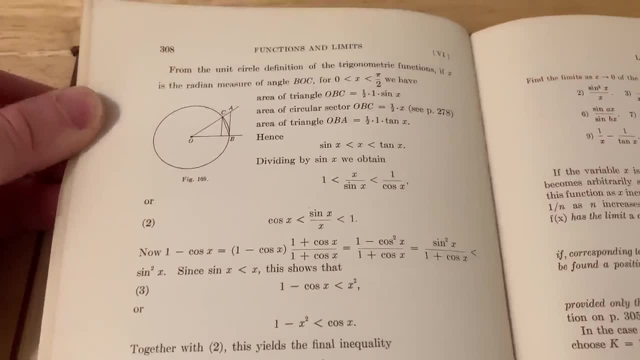 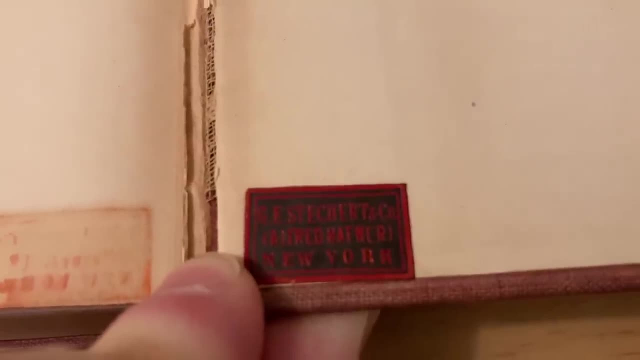 that Courant has provided in his beautiful book. I just noticed this mysterious stamp here in the back of the book. That's really cool. I don't know what that is. Yeah, wow, What an old book. Derivative and velocity. 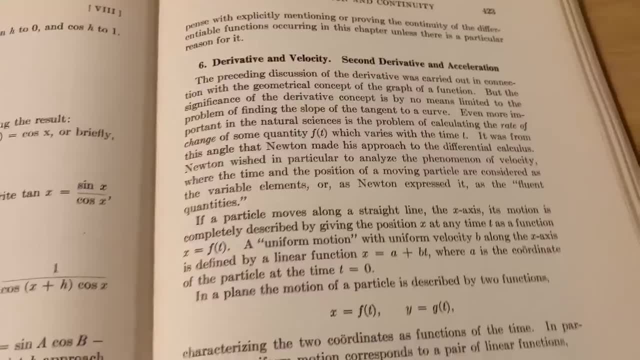 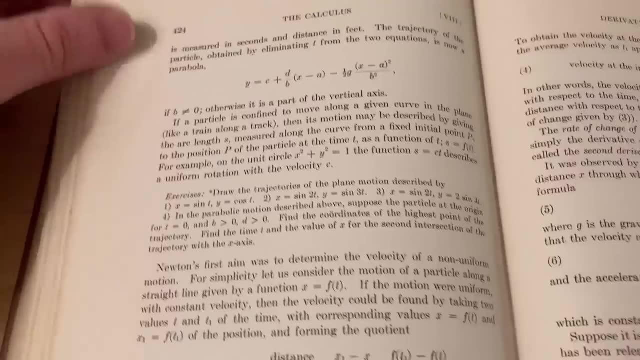 second, derivative and acceleration. This is something that is typically taught in a Calc 1 course, and so you see it again here in Courant's book, which is really cool. The amount of mathematics that this book contains is really quite remarkable. 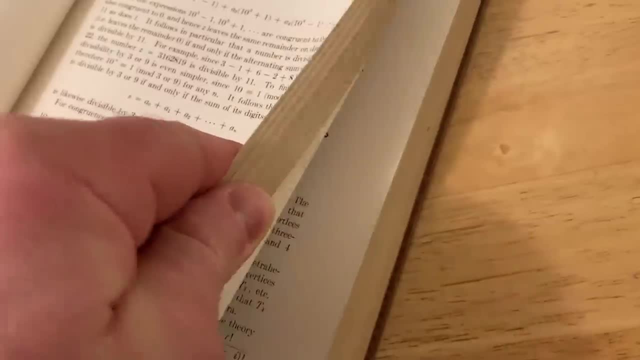 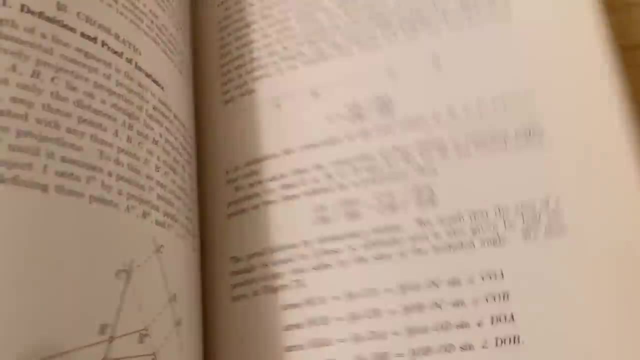 and for the thickness of the book. I think it contains an incredible amount of math. Having said that, there are sections that are a little bit more terse, and it does require some thought to read this book, but there's also no exercises. 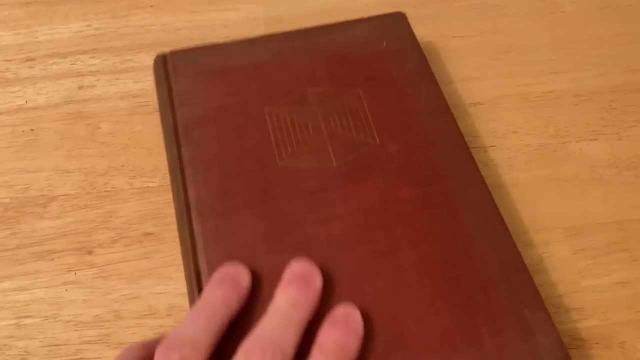 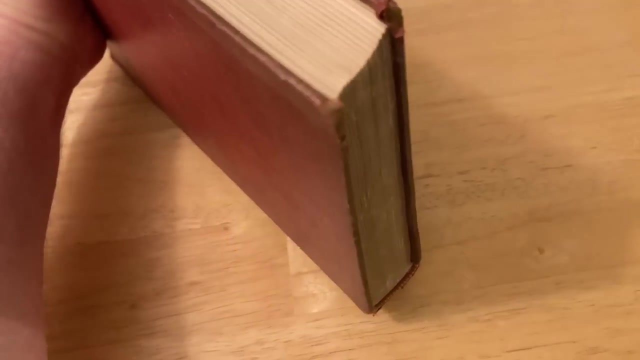 and so I think that really saves on pages. Perhaps the most shocking thing about this book for me personally is that I've realized that mathematics can be explained in a crystal clear way by some people, and I think Courant is one of those people.